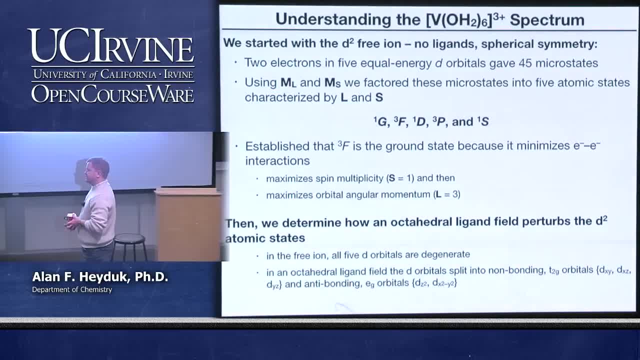 We've been talking about, or the big problem that we've set up, is how to interpret the electronic absorption spectrum and how to interpret the electron absorption spectrum. So the electron absorption spectrum is a very complex and complex structure of coordination complexes that have more than one D electron. okay, 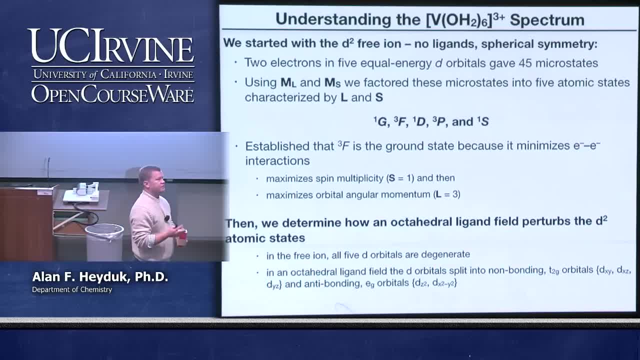 And as the prototype we looked at, we've been looking at hexaqua vanadium tricat ion, which has three electronic absorbances in the UV visible region. They can all be attributed to D to D bands. They can all be attributed to the same D to D band. 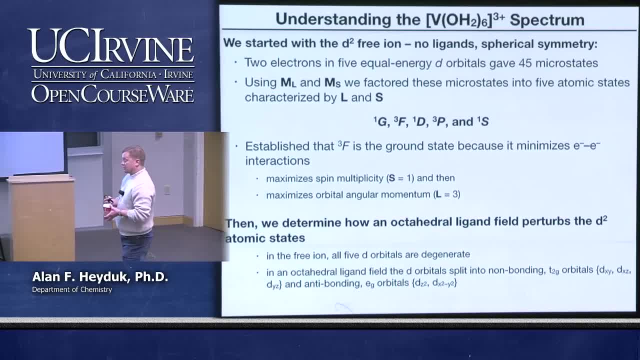 So we know that they're D to D transitions From our molecular orbital diagram. it's hard, you can't explain where the three transitions come from, And so we've been employing crystal field theory. And to employ crystal field theory you have to go all the way back to the free ion. 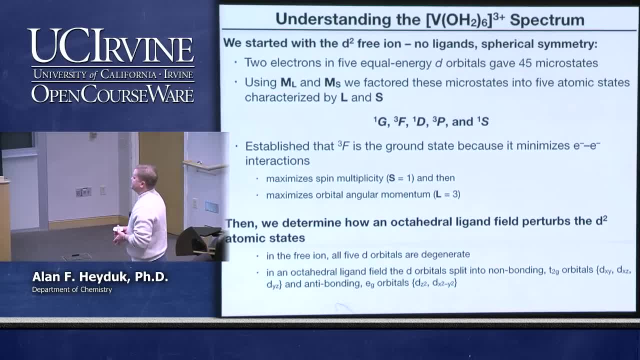 And that is when you have two electrons in five equal energy D orbitals. Now, a thing that we often forget when we draw pictures of orbitals and we put energy diagrams up in molecular orbital diagrams: all of that is based on the hydrogen atom. okay, 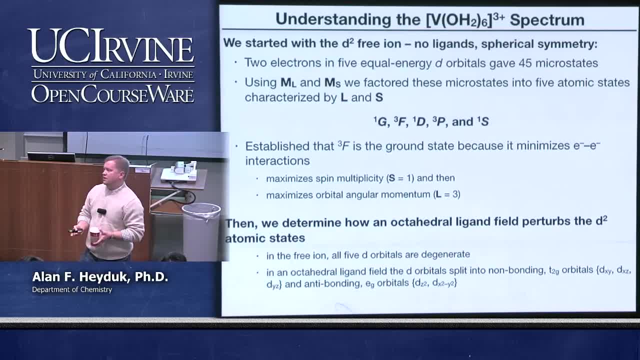 Those are all what we call one electron orbitals. okay, It's just, we can solve the Schrodinger equation for the hydrogen atom, So we calculate what a 3P orbital would look like, or what a 3D orbital would look like. 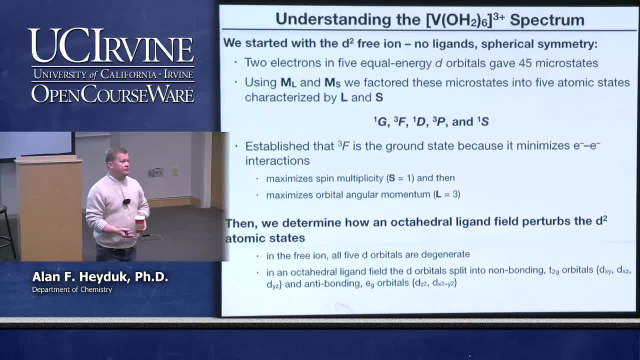 And that's the pictures that we use. okay, We can't solve the Schrodinger equation when we have more than one electron, okay, And so then that's really where this- where the issue comes up is the MO diagrams that we generate- are based. 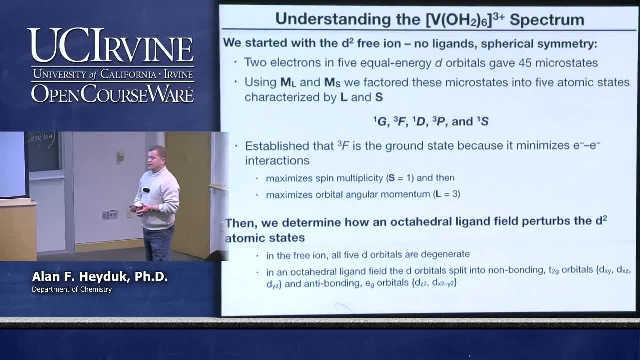 on one electron orbitals, With crystal field theory and with the spectroscopy, it gives us the ability to start to approximate what happens when you have multiple electrons in an orbital set, And so one of the things that you have to do is consider the energy. 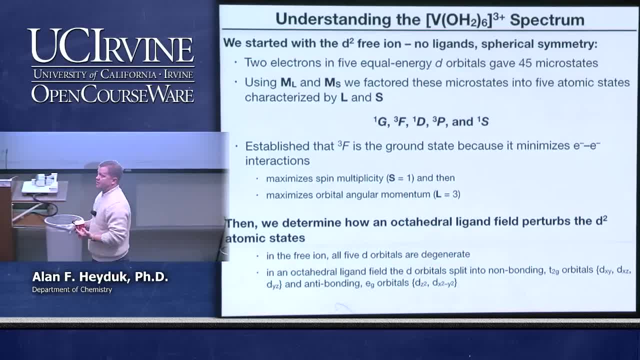 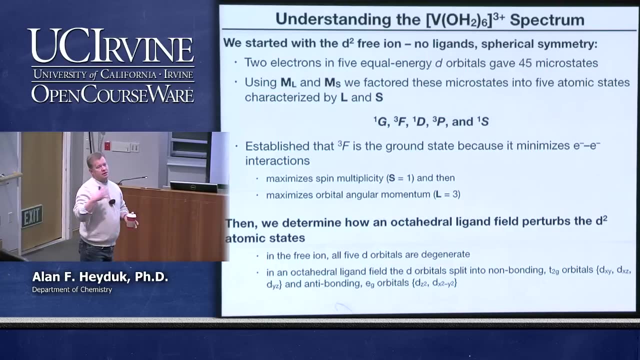 You have to consider how the two electrons interact with each other, how their orbital angular moments to couple, how their spin angular moments to couple. okay, In other words, L and S. Sometimes you have to worry about how their orbital and spin couple together. 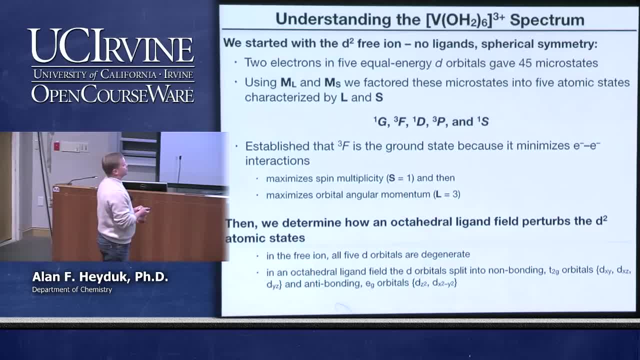 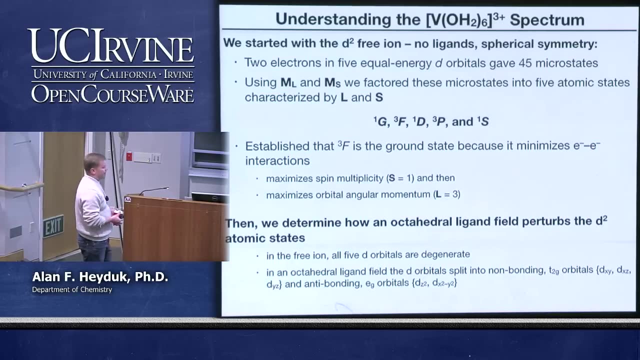 to give you J coupling, But for our purposes- we aren't going to worry too much about that- Using our big M sub L and big M sub S values. okay, So this is the. this is coupling the orbital angular momenta of the two electrons, or the spin angular momentum. 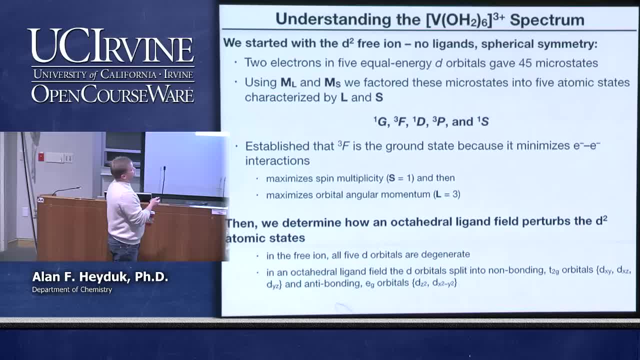 of the two electrons, We figured that the 45 microstates of the D2 ion can be factored into five atomic states. These atomic states are collections of microstates that have the same energy. So even though we have two electrons in five D orbitals, 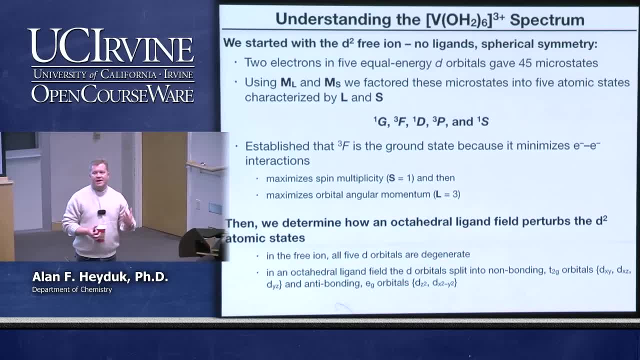 that are all at the same energy. there are. you know, there are effectively five different electronic states that are distinct. okay, We can represent them by these term symbols. Three of those atomic states are singlets. okay, So that's where the electrons must be paired. 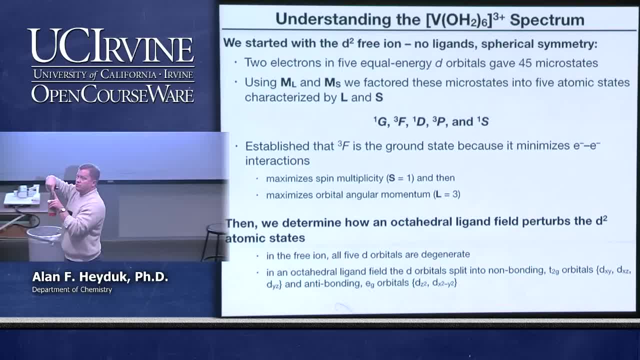 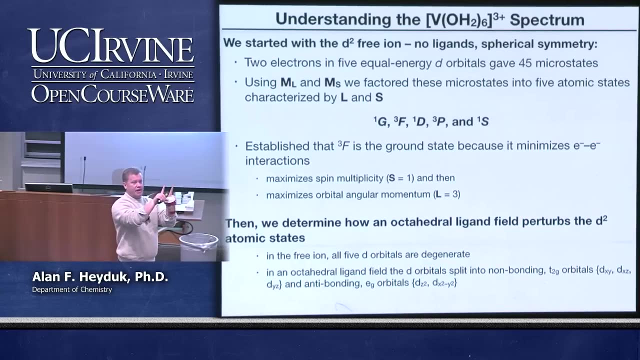 must have opposite spin, okay. So there's no, so there's a zero spin multiplicity. Two of those states, the triplet F and the triplet P, are where the electrons can be have the same spin, be pointing in the same direction, okay. 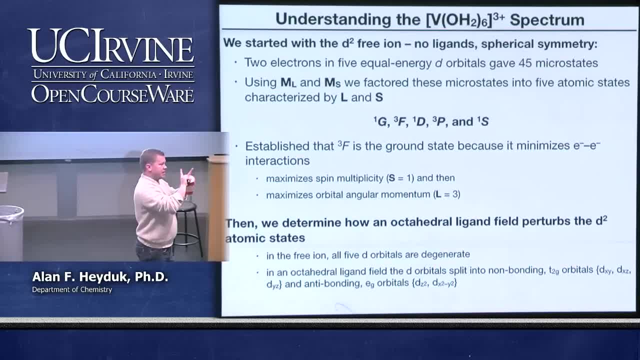 They can both be spin up, They can both be spin down. They can also. there's also a microstate where they have opposite spins in these, the triplet F and the triplet P. But the important thing is that they can have the spins parallel. 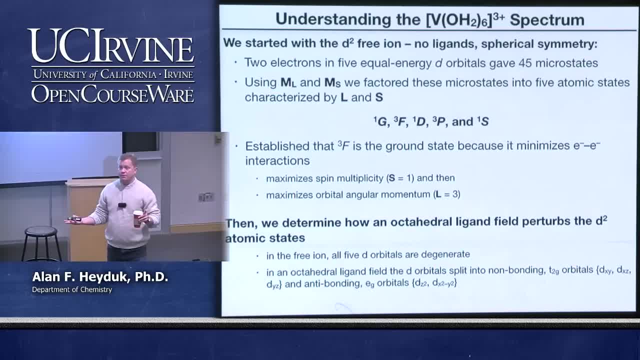 That tells you that the electrons must be in different orbitals, Because you can't put two electrons into the same orbital and have the same spin. The ground state we establish is triplet F, because it both maximizes the spin multiplicity and it maximizes the orbital angular momentum. 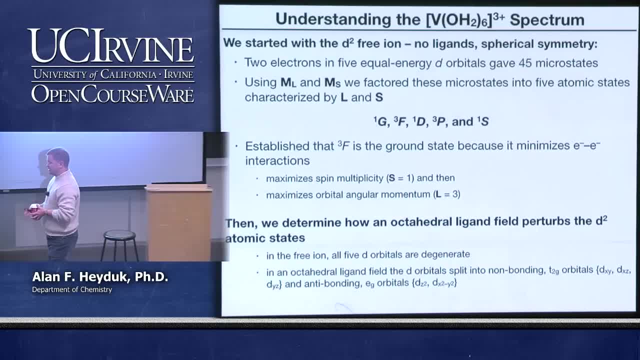 The triplet F has 21 different microstates, It's got the greatest microstate degeneracy, and it's the ground state for this molecule. So, then, our challenge? remember all of this. these five electronic states are for the free ion, where the d orbitals are all at the same energy. 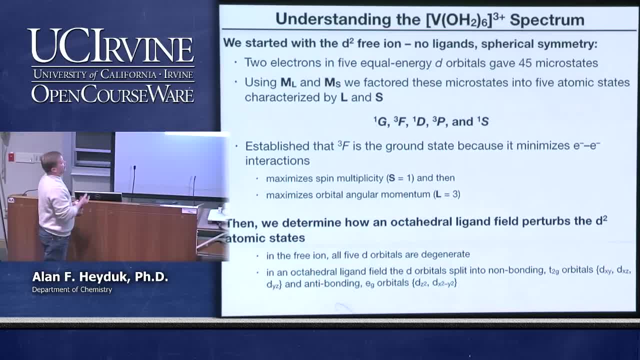 But we know for hexaqua, vanadium tricat ion that we have an octahedral complex and that the ligand field generated by these six water molecules causes the d orbitals to split into a nonbonding level and an anti-bonding level. 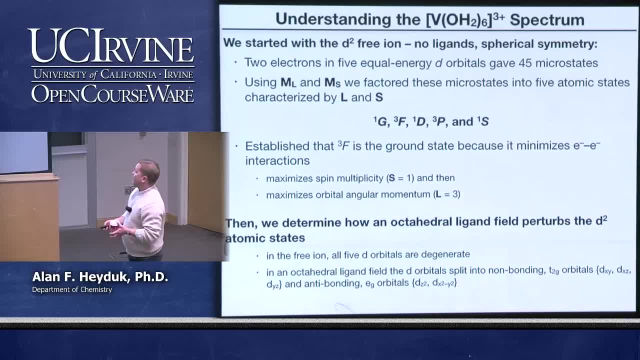 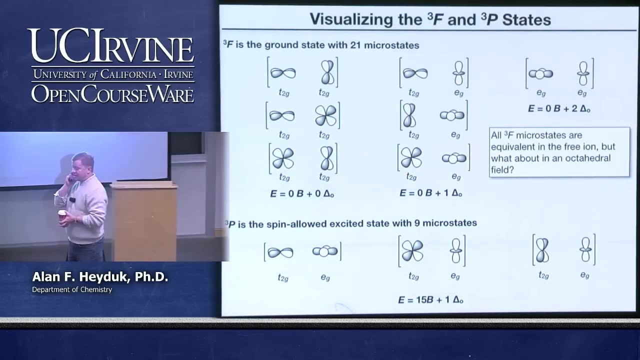 The d orbitals are no longer all degenerate, And so we have to figure out how this octahedral ligand field perturbs the energies of these five atomic states from the free ion, And so to do that, last time we went through 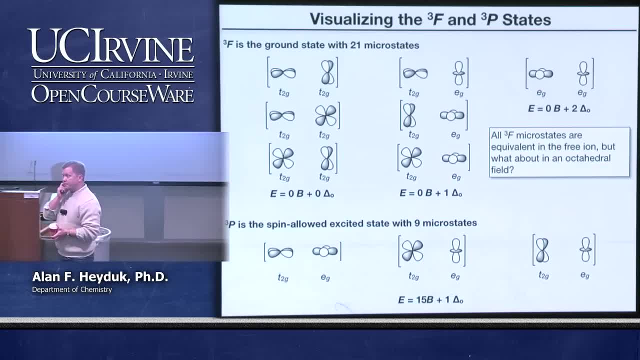 and we drew pictures. okay, And when I put together these notes, I did it in the absolute simplest way possible. I sat down and I said: I have two electrons and I have five orbitals and what are all the combinations I can have? 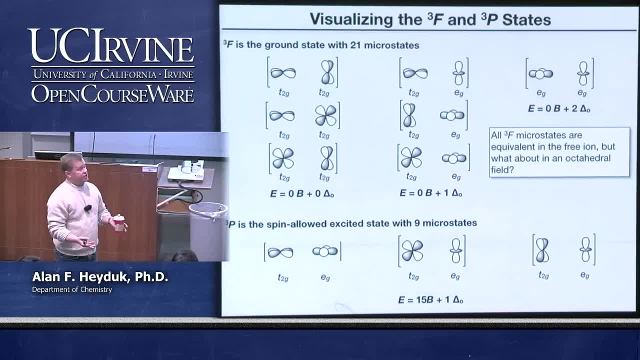 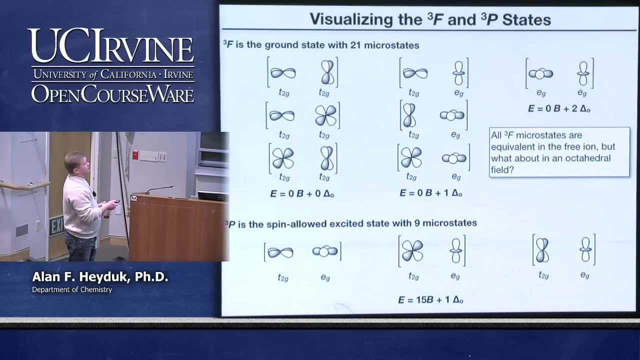 And I drew them all out and I looked at the sheet of paper and I said, okay, well, can we then figure out what the differences in the interactions are? And it becomes obvious- or it should, that seven of the orbitals are in the same place, right? 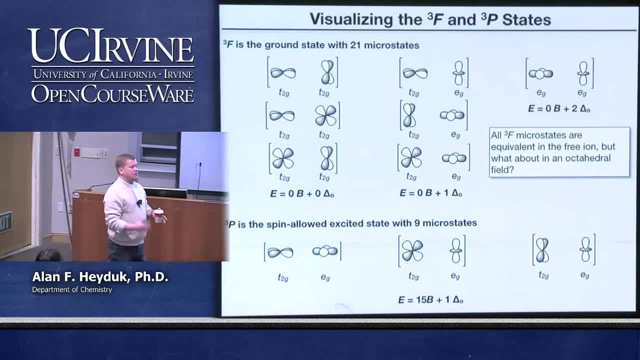 So what we can do is we can get the electrons, and the electrons are in the same place, right? So these two orbital combinations minimize electron-electron interactions by putting the electrons in different planes of the vanadium ion, right? In all of these cases, all of these micro-state, 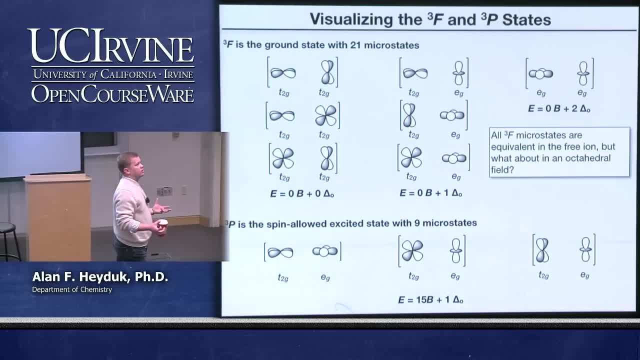 or these orbital combinations that belong to the triplet F. the two electrons of the vanadium are as far apart as possible because they're localized in different planes. combinations put those electrons in the same plane because electrons have negative charges. Putting the two electrons in the same plane. 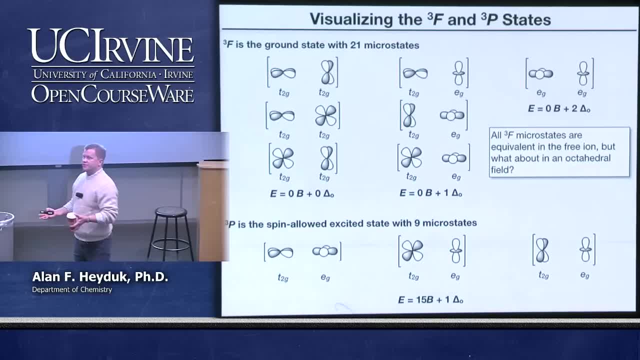 of the vanadium ion is going to cause a repulsive energy, And so these three orbital combinations make up the triplet P atomic state, which is higher in energy than the triplet F. Okay, so that's how we separate out the triplet F microstates. 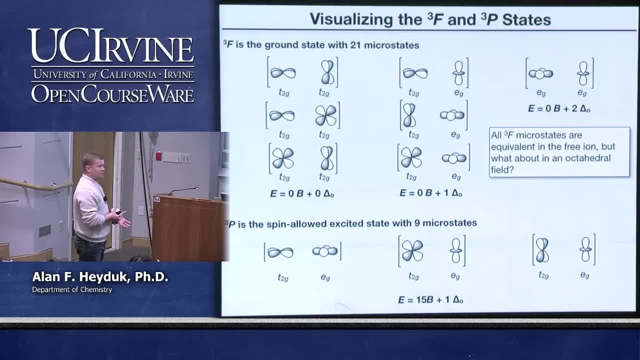 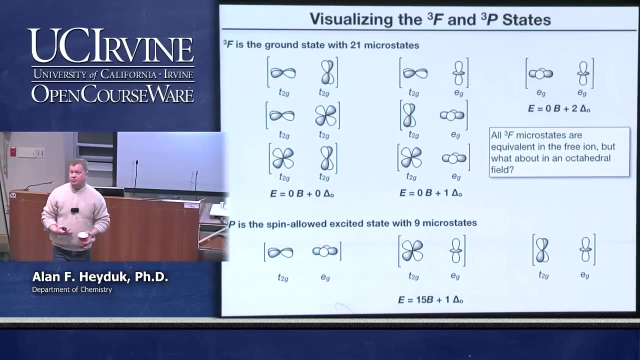 from the triplet P microstates in the free ion. The next step is to put the octahedral ligand field on top of this as a perturbation. And again, once we have these things all drawn out, it's easy to go through and say this: orbital. 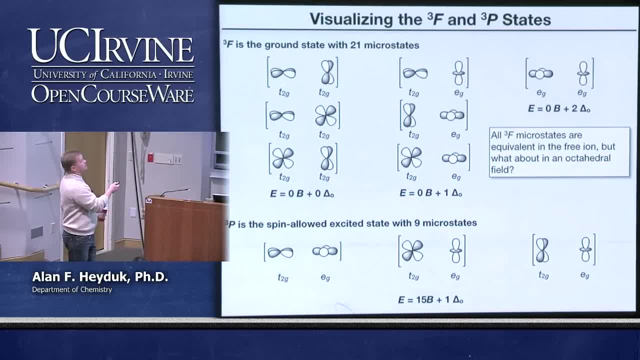 this DXY orbital belongs to the T2G. It's a nonbonding orbital. This DXZ also belongs to the T2G. It's nonbonding. And we can go through each of these seven orbital combinations, plus these three orbital combinations, and assign the character of the orbital. 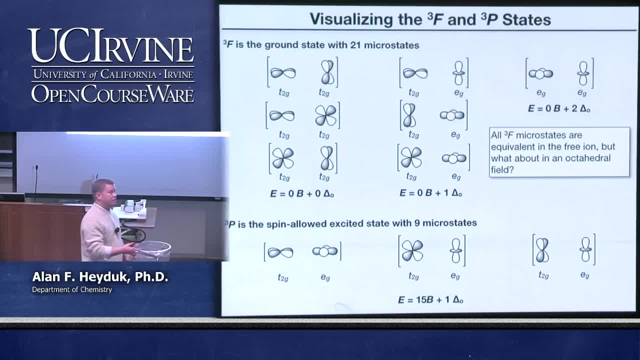 in the octahedral ligand field. Once we've done that, we can add the energy term. We can decide what energy perturbation the ligand field brings. if the orbital belongs to EG, That means an electron in this EG type orbital is going. 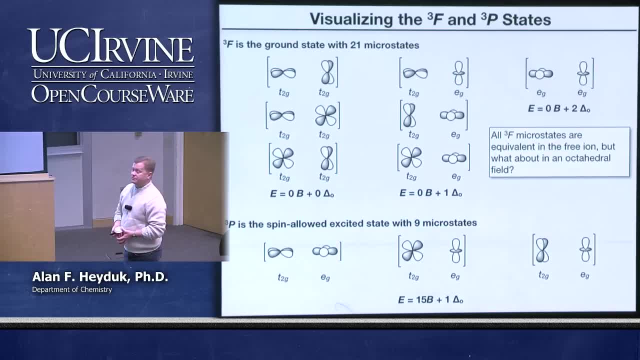 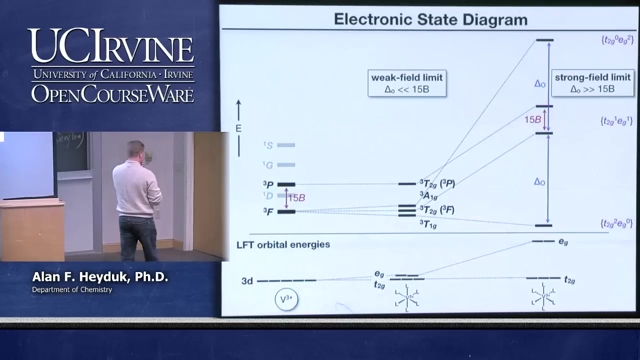 to be destabilized by delta O energy, And so we can write very simple energy equations to approximate where each of these microstates is going to be an energy once we apply the octahedral field, And so that led us to this diagram. On the far left of the slide we have the so-called free ion. The vanadium tricat ion with two d electrons- I guess I should have put the electrons in there, but with two d electrons gives rise to five atomic states. The difference in energy between these atomic states is just electron-electron repulsion. 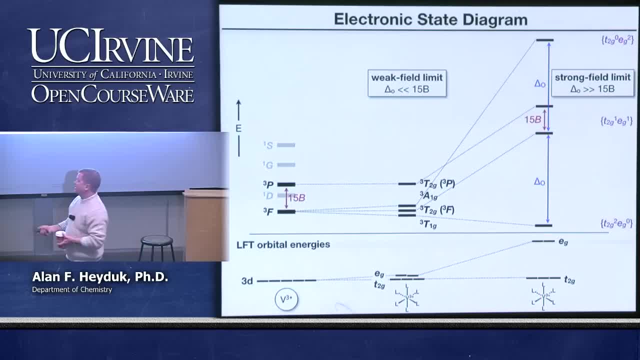 All the d orbitals are at the same energy, So the only thing that separates the triplet F from the triplet P is that repulsion associated with putting two electrons in the same plane of the ion. You can make similar arguments about the energy of this singlet D, the singlet G and the singlet S. 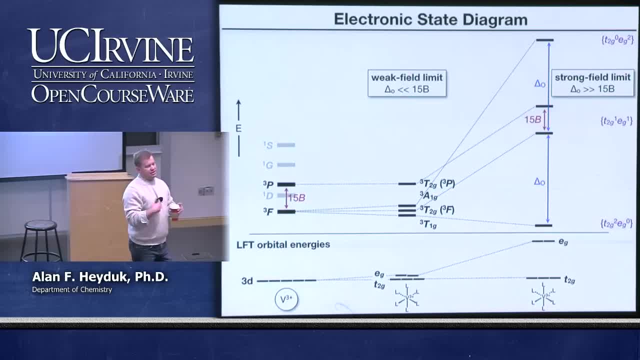 So we're going to do that. So we're going to do that For those. it's not just the plane that the electron is oriented in, but you actually have pairing energies, where you can put two electrons into one orbital. But all of these energy separations are just electron-. 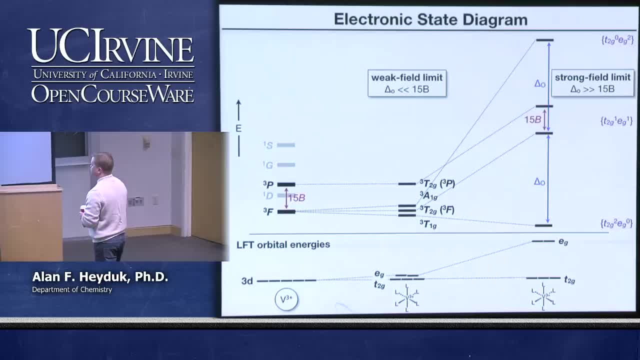 electron repulsion. due to electron-electron repulsion, As soon as we introduce a ligand field, as soon as we go from spherical symmetry to octahedral symmetry, the d orbitals become inequality. DZ squared and DX squared minus Y squared make up the EG. 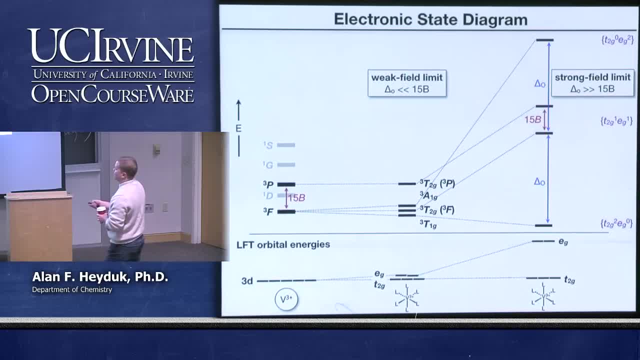 XZ, YZ and XY make up the T2G. They're going to be at different energies. The EG is going to be higher. But this middle position right here is what we call the weak field limit. We have an octahedral field. 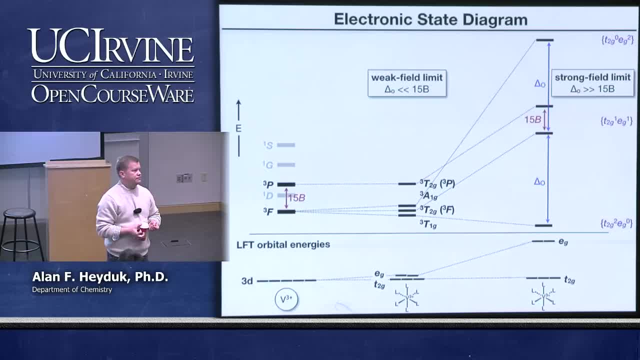 But the value of delta O is very, very small. Okay, We can say it's almost zero, Just enough that we can see the difference in the energy of these two levels. When we introduce this octahedral ligand field, it breaks the symmetry. 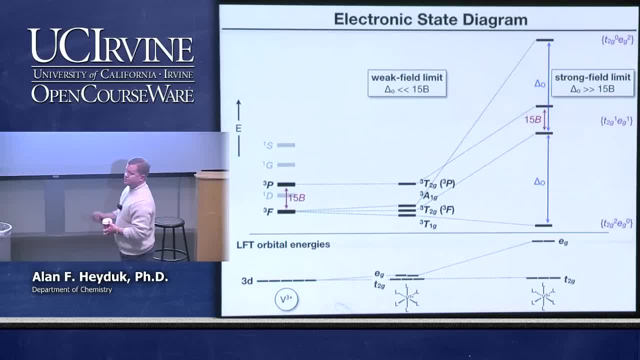 Okay, Spherical is the highest symmetry we can have. Going to an octahedron breaks that delta. Okay, So we're going to have a very, very small energy. So we're going to have a very, very small energy. 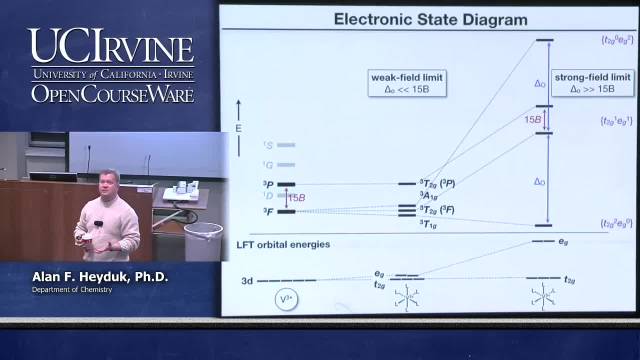 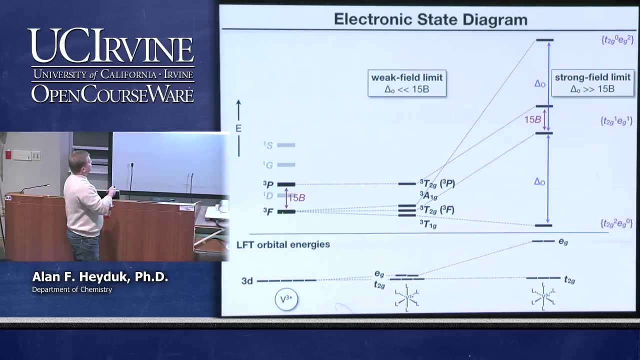 It's cubic. It's still a very high symmetry, But it's less than spherical. Okay, Just like the d orbitals are, no, just like the fact that these are no longer degenerate once we go to the octahedron, the two triplet states break. 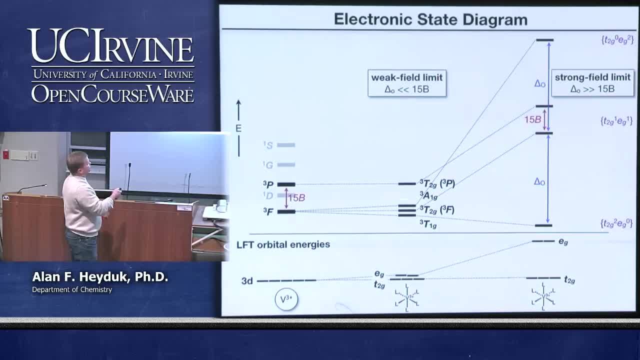 down because of the symmetry. The triplet F decomposes into three different states. A triplet F decomposes into three different states: A triplet T1G, a triplet T2G and a triplet A1G. The triplet P actually comes across. 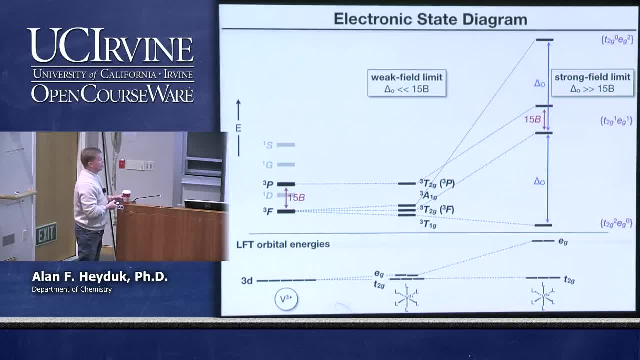 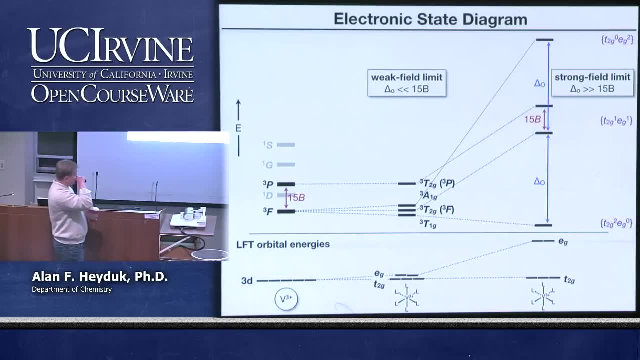 and maintains its triplet T2G configuration. Your textbook talks about how to get these labels And they correspond to the way that we put electrons into the octahedron And there's a very nice way to get those labels into these molecular orbitals. 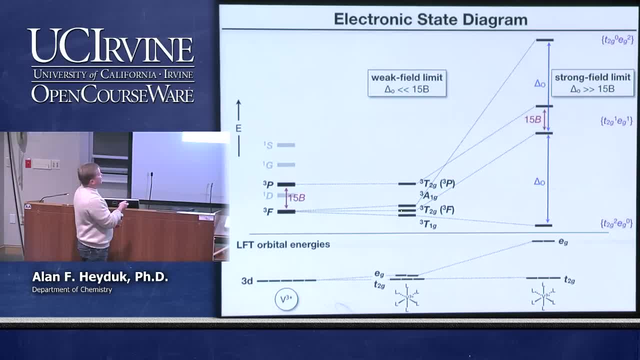 Now you'll notice here that I kept the three electronic states that came from the triplet F. I kept them very close in energy, Much lower in energy than this triplet T2G. That's because the splitting here is still very small compared to electron-electron repulsion. 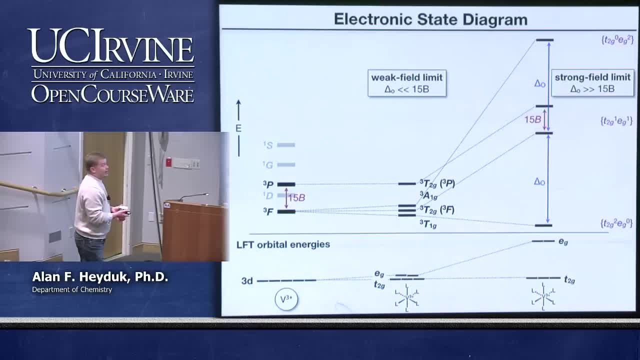 That's because the splitter here is not very large, So you don't have a big difference. That's not always the case, though. In fact, usually the ligand field imposes a greater energy, has a greater energy perturbation than electron-electron repulsion. 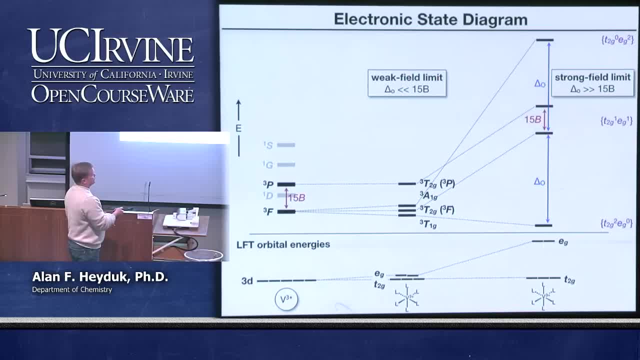 And so we can come over here to the right side of the diagram, and this is the strong field limit. On the right side of this diagram we would say that delta O, the splitting between T2G and EG, is large, much larger than the electron-electron. 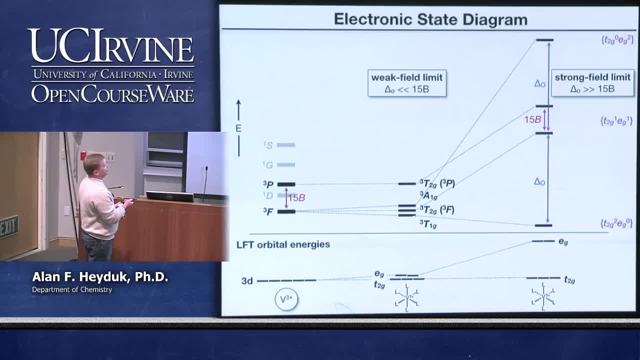 repulsion term. And so what we see now is that one of these electronic states from the triplet F basically stays low in energy, stays the ground state, this triplet T1G, One of the states, the triplet T2G goes up. 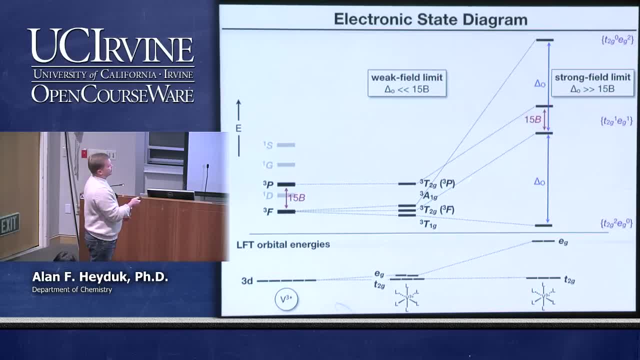 You see a, basically a one for one increase in the energy of this state with the energy of the EG orbital because again, or because this state corresponds to having one electron in EG and one electron in T2G, The triplet A1G that came out of the triplet F free ion state goes. 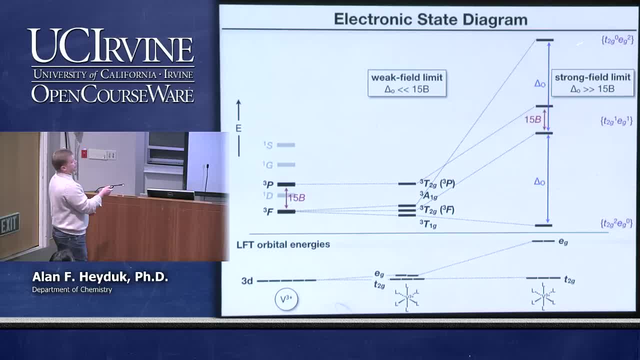 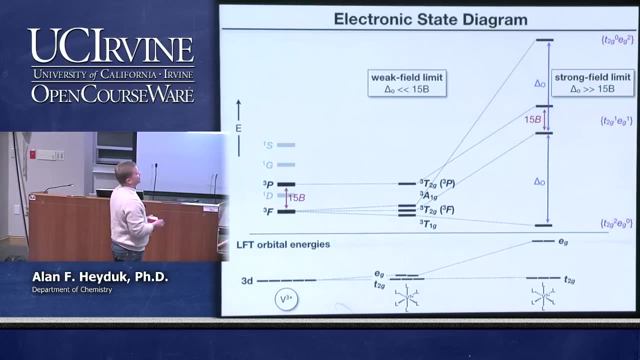 up twice as fast, so that in the strong field limit it's the highest. So that's the triplet A1G, It's the highest energy state and we can look at the electron configuration of that state: Zero electrons in T2G and two electrons in EG. 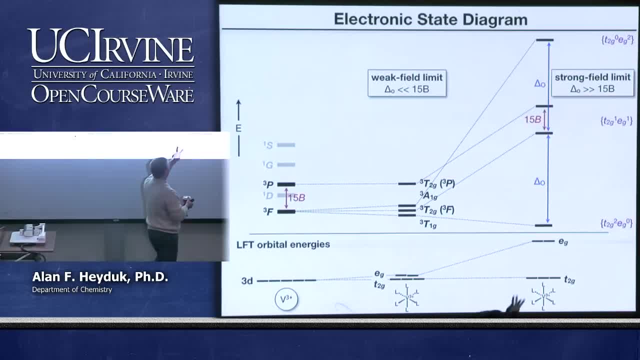 Effectively, that triplet A1G state is when you have both electrons up here in EG. The energy of that state, therefore, is going to be two delta O. Finally, you have the triplet T2G that came from the triplet P free ion state. 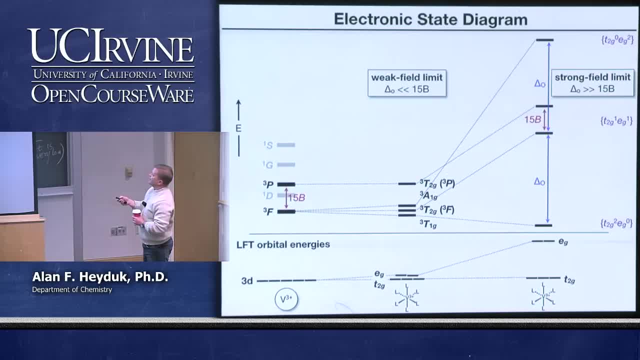 You'll notice that it also goes up. It actually parallels the triplet T2G from the triplet F atomic state. It goes up one for one with the increasing ligand field strength so that when we get to the end the strong field limit here. 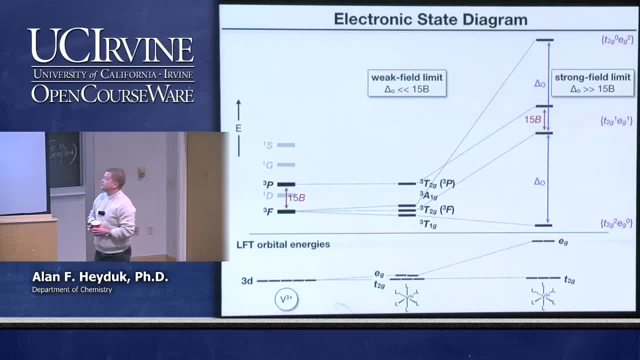 it's exactly 15B higher in energy than the triplet T2G. So that's the triplet T2G from the triplet F free ion state. The exact same energy separation of the triplet F and the triplet P in the free ion. So what we end up with, what this is telling us, is 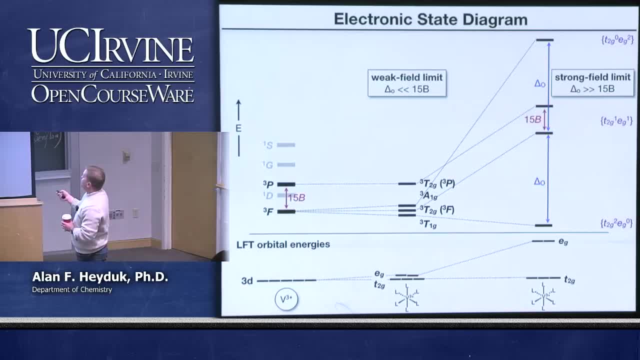 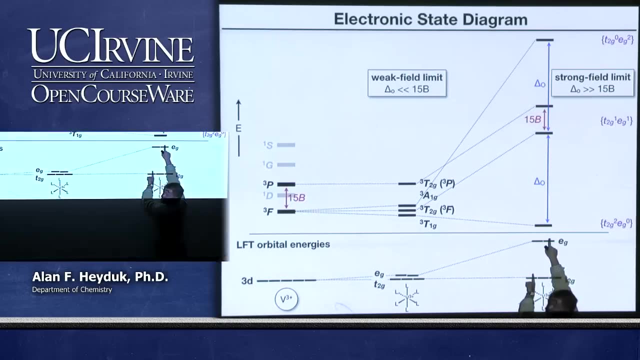 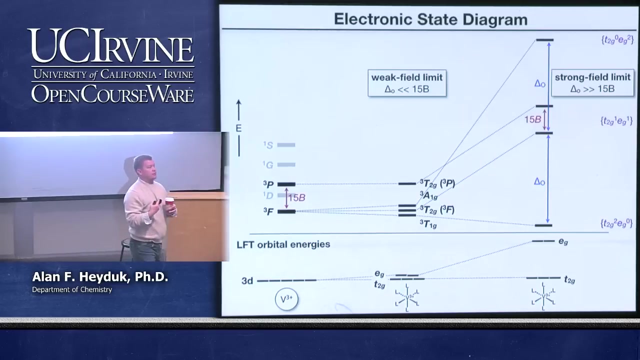 that we have two electronic states. Both of these electronic states have an electron configuration that contains one electron in T2G and one electron in EG. In other words, both of those states correspond to this. It just depends on whether you also include an electron-electron. 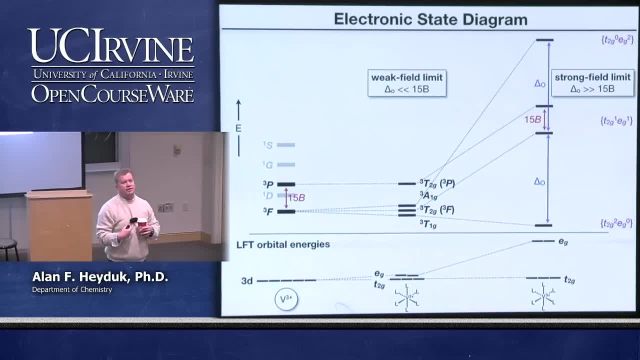 repulsion term because the electrons are in the same plane. So if the specific configuration, if the specific microstate is to have an electron in XZ and an electron in Z squared, that configuration puts the electrons in the same plane. It's part of that state that triplet T2G derived. 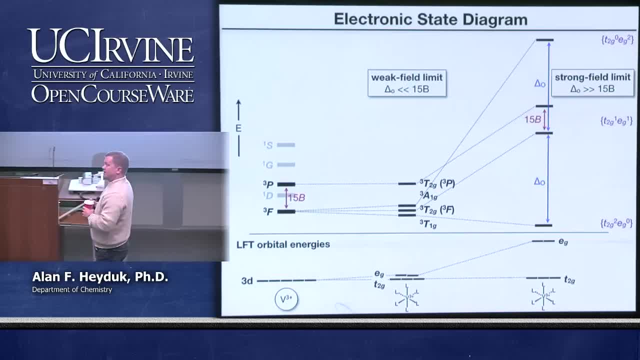 from the triplet P. If the specific microstate has an electron in XY and Z squared. well, that's different planes. That specific microstate or electron configuration belongs to that triplet T2G, The one that would be in the same plane. 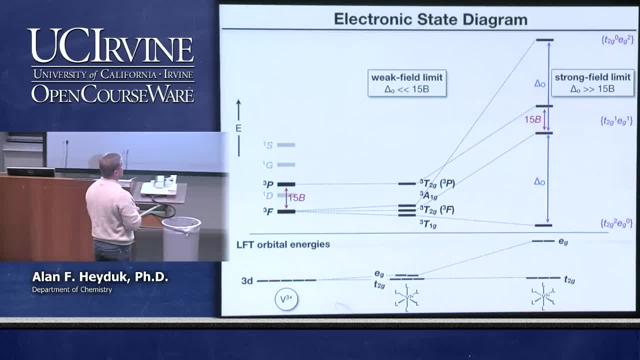 That was derived from the triplet F, And so two notable things come out from this diagram. First of all, we know that we have this triplet T1G ground state. OK, That again corresponds to the different ways that you can put two electrons into this T2G orbital. 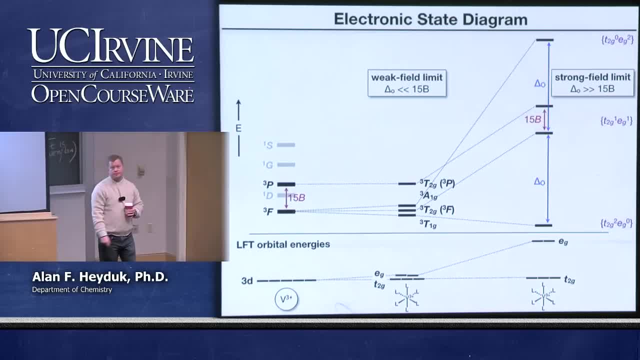 There's basically three different combinations. OK, That's going to be the ground state. That's no surprise. From that ground state, though, look, we have one, two, three different excited states, three different possible electronic transitions. that corresponds to the three different photon energies. we. 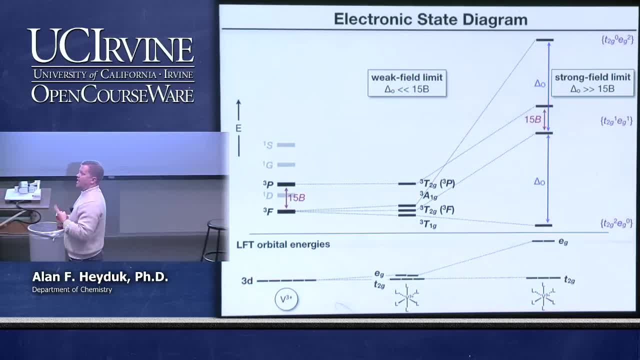 measure in the UV visible spectrum of the hexaqua vanadium ion. Those three transitions correspond to one, two, three excited states that exist in this molecule. It's kind of neat. The lowest energy transition we can predict is a direct measurement of delta O We can. that's a good approximation. 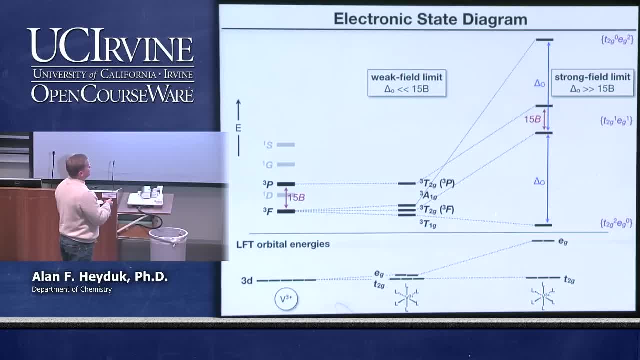 The second transition from the ground state to the second excited state is delta O plus 15B the energy of the electron-electron repulsion. The highest energy transition should be exactly or exactly or fairly close to twice the lowest energy transition, because it's two delta O. 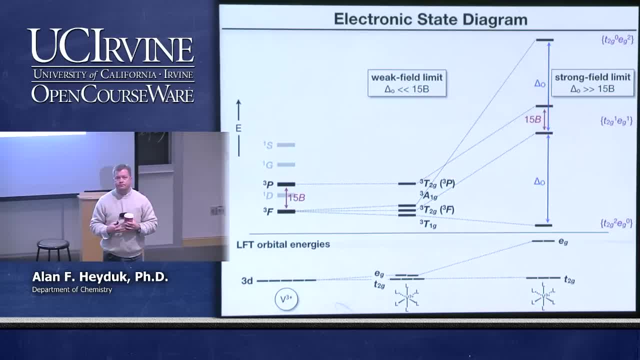 Now it turns out that every D2 ion in an octahedral field will have an electronic state diagram that looks just like this. It doesn't matter what the metal is, It doesn't matter what the ligands are, If it's a D2 ion in an octahedral field. 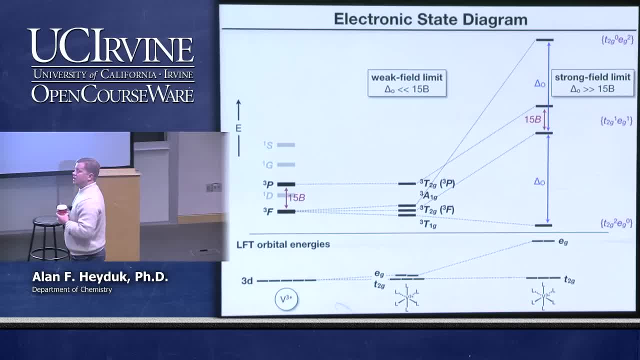 it will look just like this. The only things that change are the magnitude of B- okay, because it's going to depend on the size of the metal- and everything else- and delta O, the octahedral ligand field splitting, because that depends. 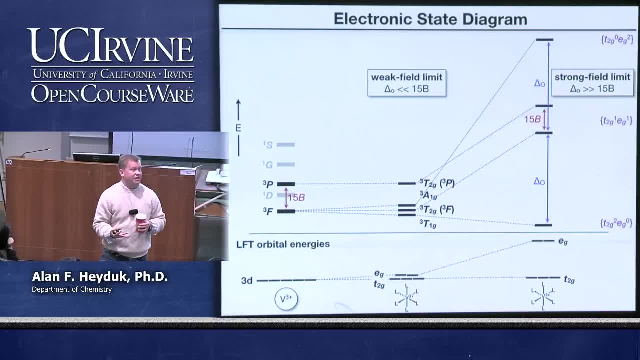 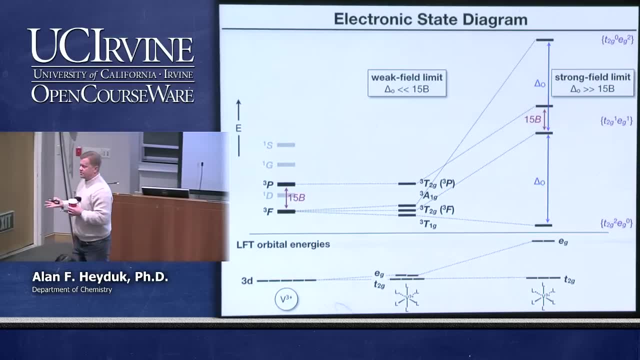 on both the metal ion and the nature of the ligand that comes in. So to accommodate the fact that the basic diagram doesn't change, but just the magnitude of these energies. the magnitude of these energies doesn't change. it's going to depend on the size of the metal and everything else. 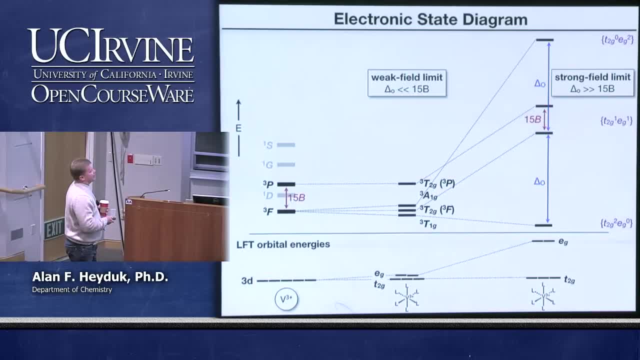 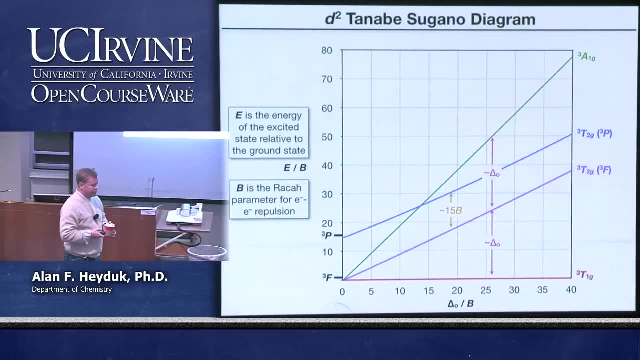 But if the magnitude of these energies does change, you'll often see these state diagrams collected in what's known as a Tanabe-Sugano diagram. So first things first. in this Tanabe-Sugano diagram, I'm only showing the triplet electronic states. 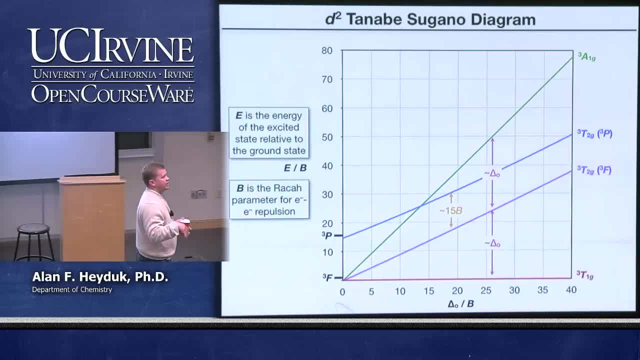 I've just gotten rid of all the singlet states, because we know that we can't see those states spectroscopically because it requires a spin flip. So over here. well, let's start on the x-axis of the Tanabe-Sugano diagram. 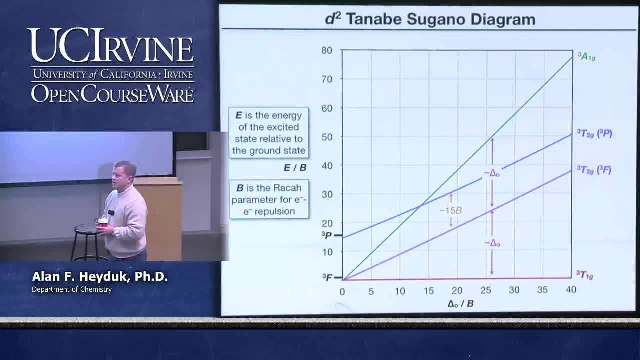 We have the value delta O over B. So the x-axis gives you the octahedral ligand field splitting or the crystal field splitting in units of B. Okay, we effectively delta O is going to be a measurement in energy. 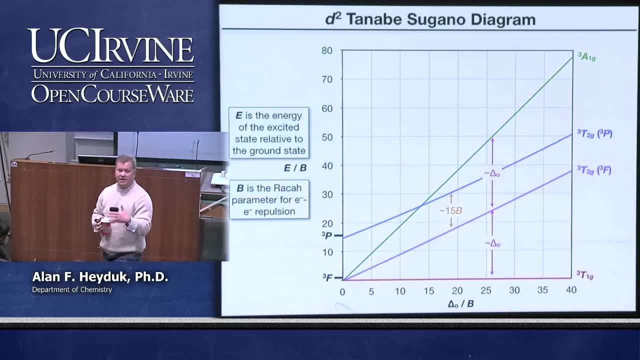 B is going to be a measurement in energy. If we divide delta O by B, we cancel out our energy units and we're left with a scale that runs from 0 to 40.. The y-axis: we have energy divided by B, The E in this case. 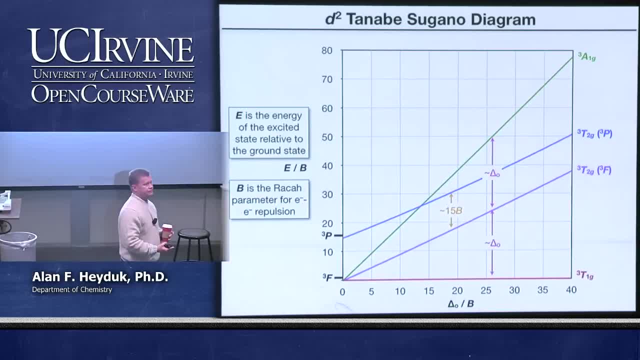 is the energy of the electronic transition. It's the energy that you measure from your spectroscopy. It's the energy that you measure from your spectrometer, Not the wavelength, the energy. Okay, Again, we divide it by B so that we get rid. 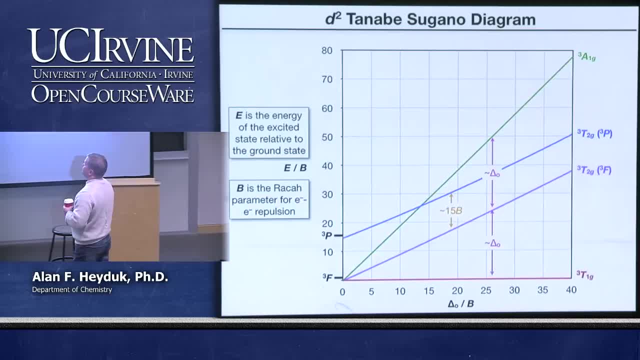 of whatever energy units we're using, and we get a scale, a scalar on the y-axis to go along with our scalar on the x-axis. So now it should make sense to you that if we come along here on the x-axis down to a value, 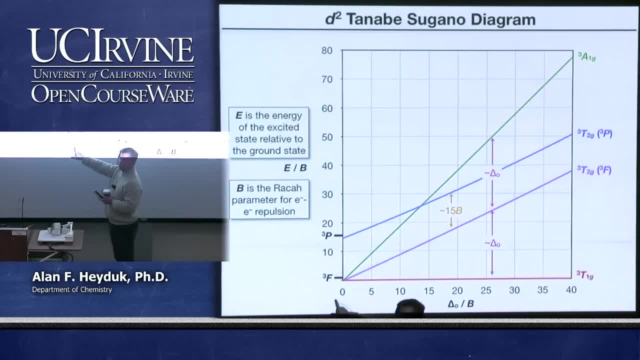 of delta O over B equal to 0,. well, that's telling you that delta O is 0. It's effectively the free ion. There's no octahedral ligand field, And so at 0, we put our triplet F as the ground state. 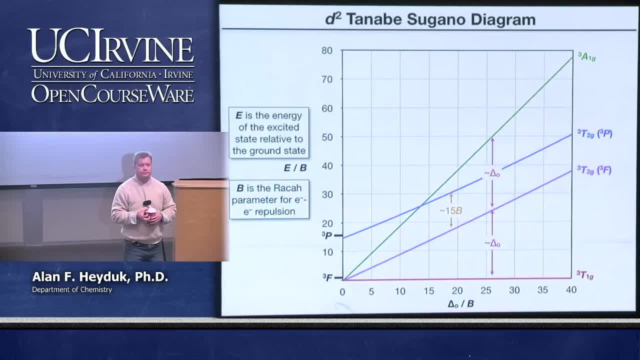 and our triplet P as the excited state, That separation- if you excuse the fact that that got shifted a little bit- that triplet P, that separation between the triplet F and the triplet P is exactly 15B As we move from left to right along the x-axis. 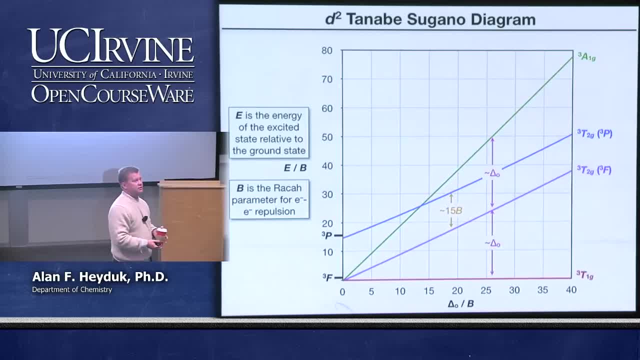 we're increasing the strength of the ligand field, Delta O is becoming larger And what we see happen is our triplet F splits into three electronic states: The triplet T1G, which we normalize so that it's always 0 because it's always the ground state. 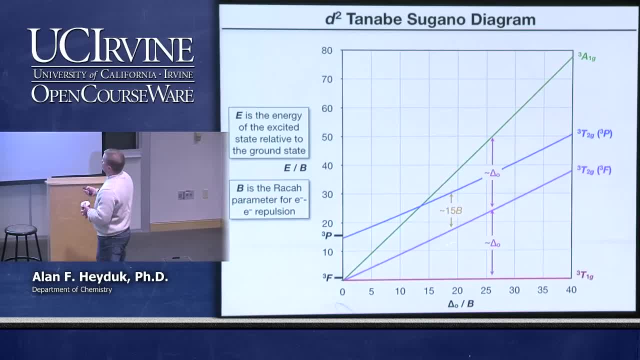 We have our triplet T2G in purple here. Okay, this is the state that corresponds to one electron in T2G and one electron in T2G. So we have a triplet T1G, We have a triplet T2G. 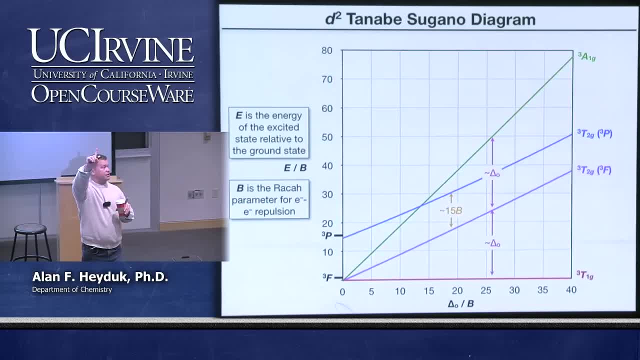 We have a triplet T2G. We have a triplet electron in EG, but so that the electrons are in different planes. And then the green is the triplet A1G. That corresponds to both electrons being promoted up to the EG orbital. You'll notice that this purple line is a one-for-one increase. 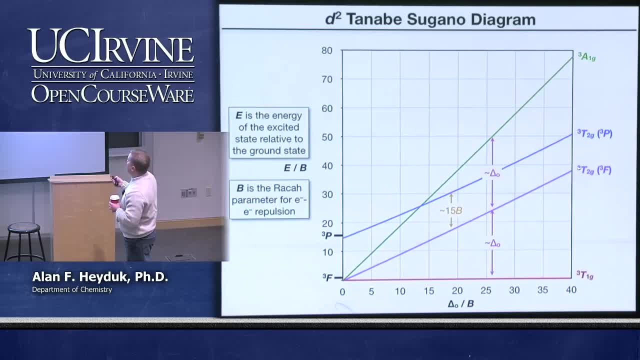 or close to a one-for-one increase. It's a line with a slope of one. This separation between the ground state triplet T1G and this triplet T2G is always delta O. Similarly or analogously for the triplet A1G, the slope of this is about two. 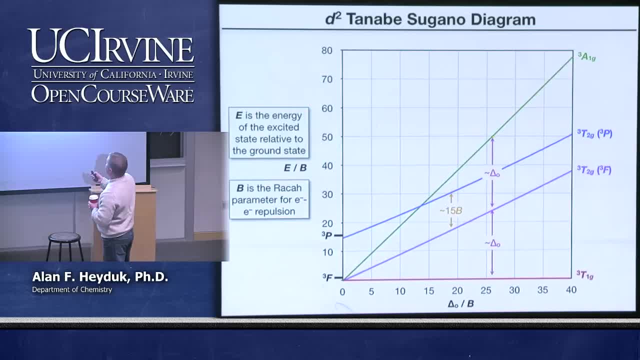 And the separation from the ground state to the triplet A1G is always approximately two times delta O. Okay, So we have our triplet A1G. The triplet P, free ion state, as we said on the last slide, stays together as a triplet. 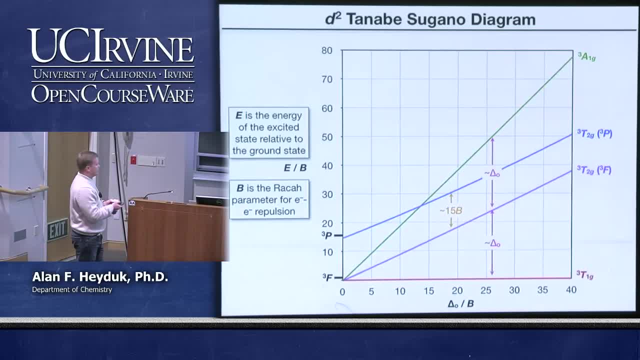 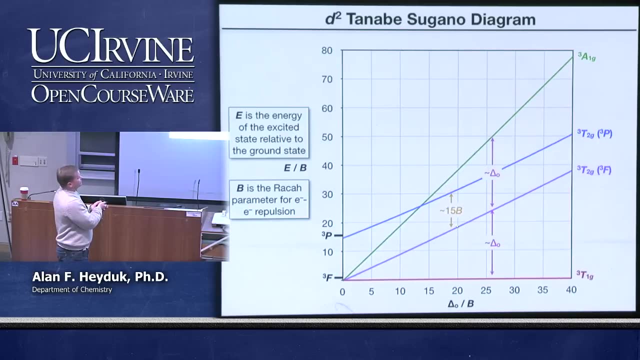 and becomes a triplet T2G in octahedral symmetry. Again, this electronic state corresponds to an electron in T2G and an electron in EG, just with the electrons in the same plane. So it's always three times T2G. 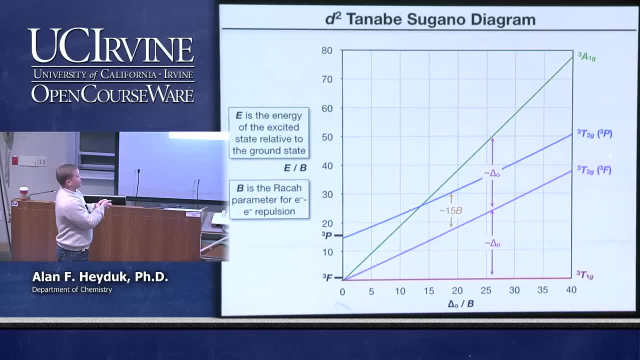 Fifteen B higher than the purple state. Yeah, Why did you choose to measure delta O after 25?? Delta O is already. Oh no, I'm just showing you. I mean that was just to make the slide look pretty. 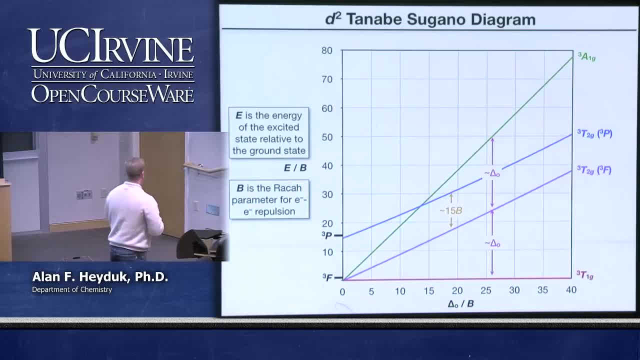 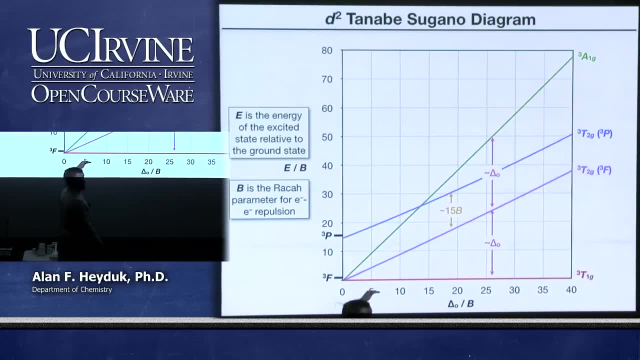 Then so does it. does delta O change? What's delta O changing? Delta O across the bottom is change. That's what the X axis is Okay. That's what the X axis is right. We're effectively taking delta O in units of B. 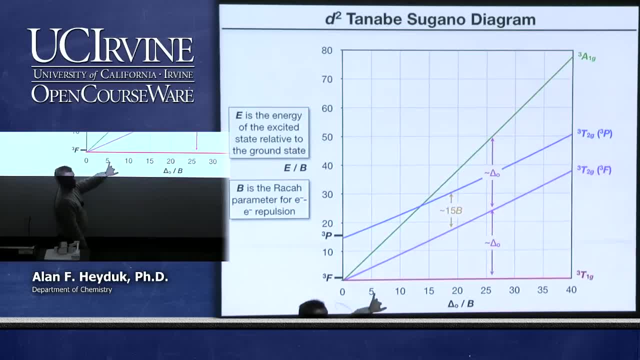 So if delta O is five times B, then it's here. If it's 25 times as large as B, then we're here. Okay, So that's the X axis. That's the beauty of it is it gives us the sliding scale. 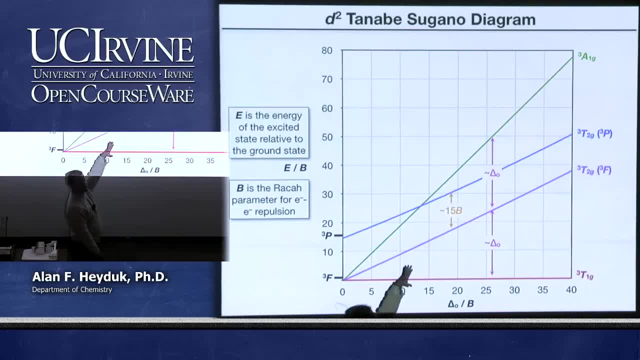 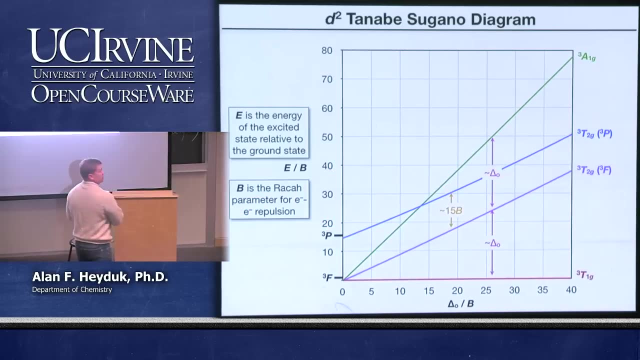 of delta O. It shows what happens to the separation between the states as delta O gets five times larger than B, 10 times larger than B, 20 times larger than B. Okay, But everywhere along this X axis you can measure a delta O value. 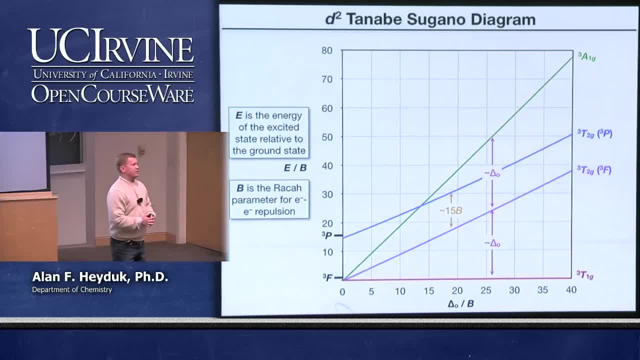 It's just a delta O in units of B. So like when you said, this is generic for all D2.. So if you just measure the B of a various D2 ion, then you can find its. So we're going to go through a sample problem. 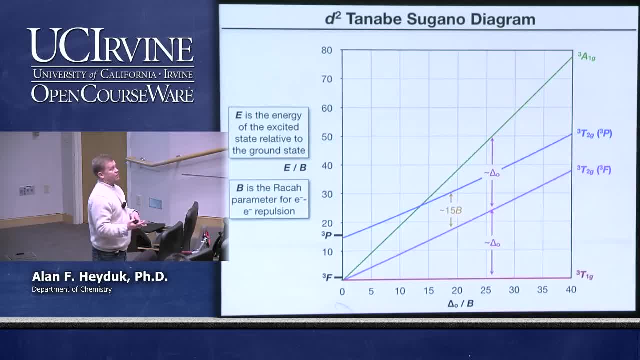 where I give you a delta O And I give you a B value And we calculate where the electronic transitions should be. More normally, what would happen is you would make a complex, You would measure its electronic absorption spectrum And you would have three transitions. 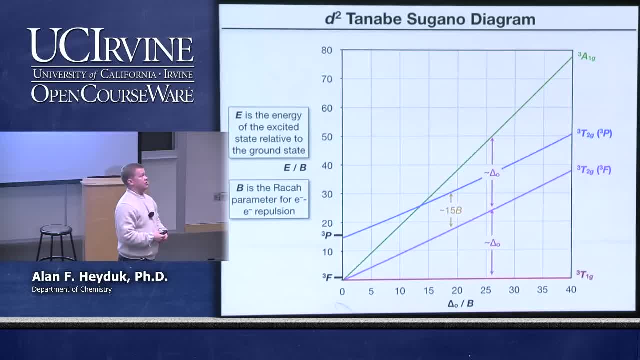 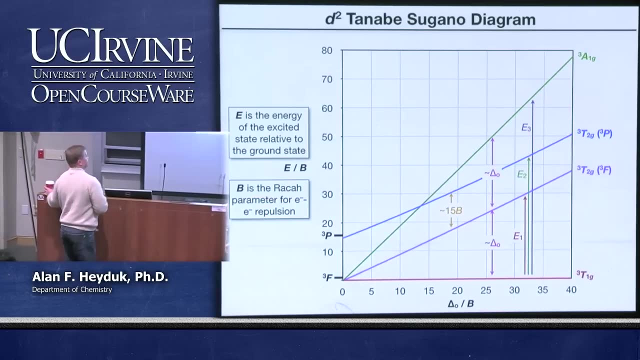 And you would have to work backwards to get and you'd solve delta O and B. Okay, So we can see now from this Tanabe-Sugano diagram if this red line, okay, this value where E over B is equal to zero, is the ground state. 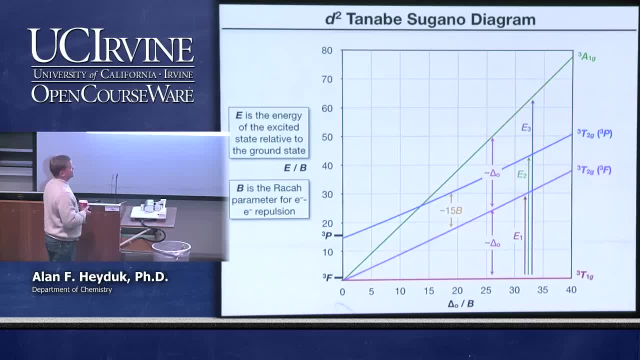 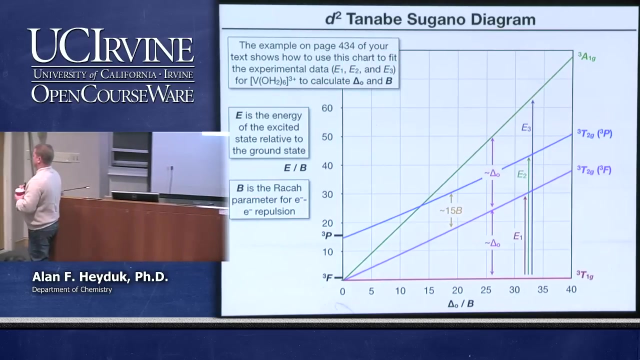 We can see very readily how we get three different transitions: to the first excited state, to the second excited state or to the third excited state. It's kind of an unfortunate color choice there. So page 434 of your textbook, I think that's the up-to-date page. 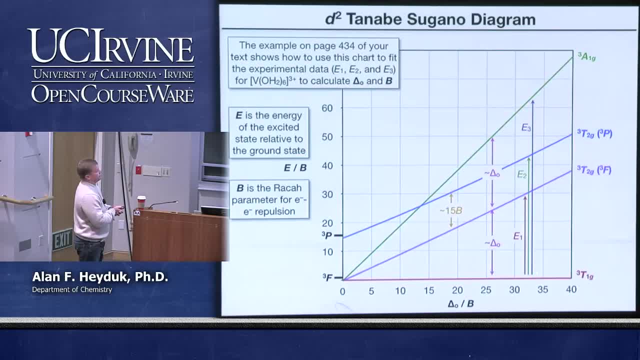 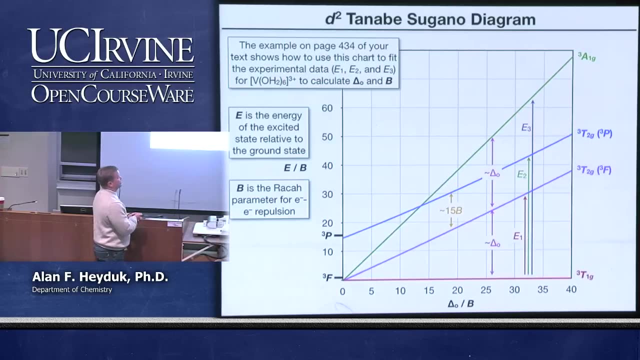 shows you how to go through and fit, when you have these, These three transitions, how to go through and fit the data and figure out exactly how to calculate delta O and B based on these three transitions. You basically have to play a trick, Okay, Which is to take two, the energies of two transitions. 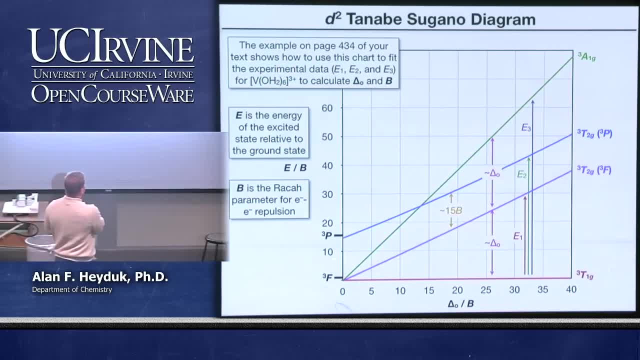 and take a ratio of them, And it would be, And it will tell you where on this sliding scale of delta O over B you are. When you take that ratio, you have to be clever. You cannot take the ratio of E3 to E1 because 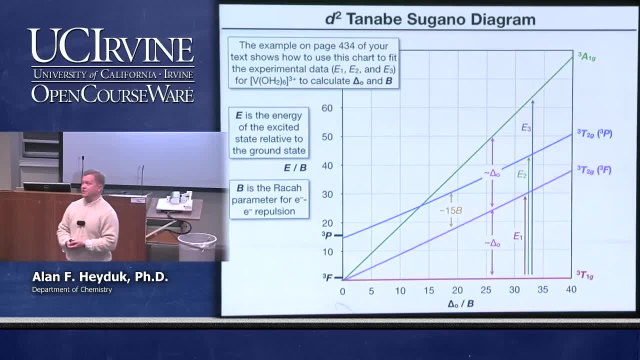 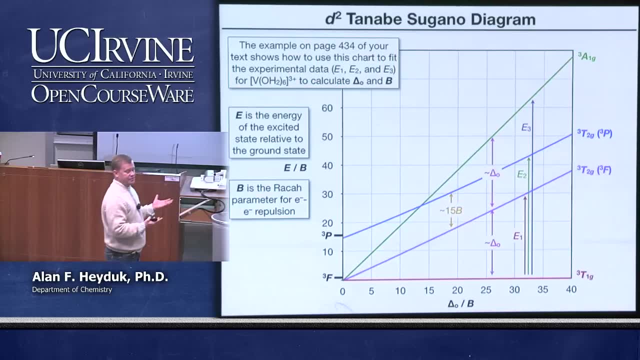 as the diagram shows, that's, that ratio is always going to be two. right, You basically are going to have two delta O divided by delta O. It's always going to be two. But if you take the ratio of E2 to E3, that one will give you. 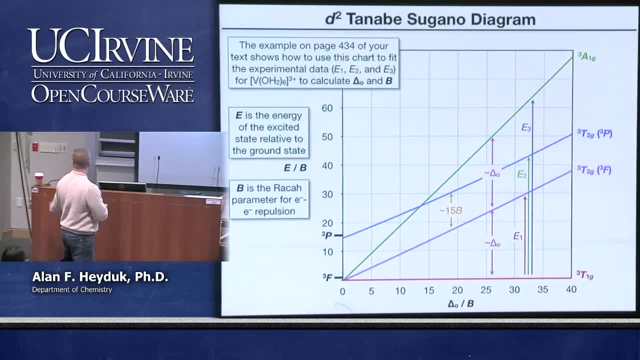 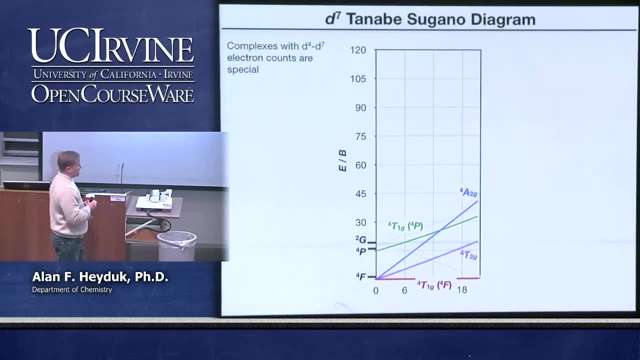 that one changes as you go across the diagram Again, your book will work you through the problem. Oh, I thought I actually had it. Oh, I have a different problem coming up. We'll come back to a different sample problem after this slide. 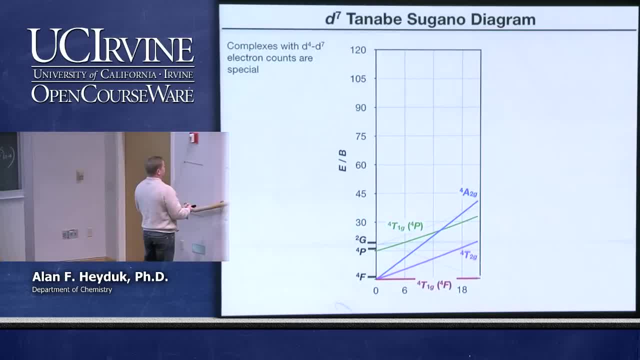 Okay, So we're going to go back to the diagram. Okay, So that was D2.. I hope it's obvious to you why we ended up with three electronic transitions. D2 is pretty much the simplest of the multi-electron states. 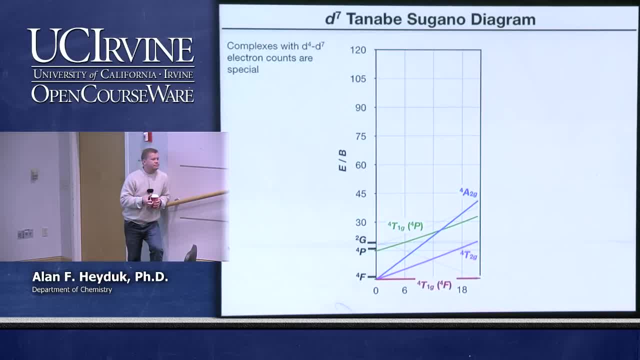 D3 isn't much more complex. It's a little bit more complex, a little bit less obvious, but it's still fairly straightforward. It turns out that D8, D9, D9 looks just like D1. There's only one possibility, one hole that can move. 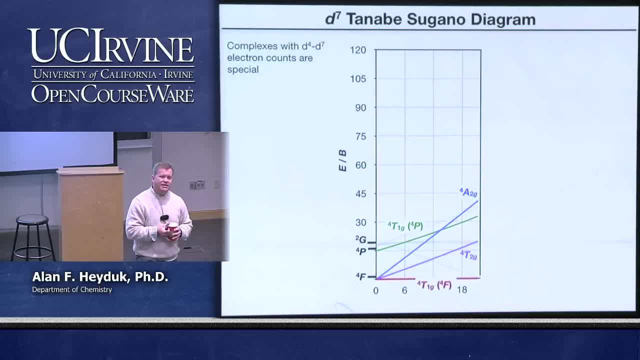 D8 looks just like D2.. D4 through 7, they kind of suck right, If you remember. D4 through D7, those are the electron counts. where you can, the complex can either be high spin or low spin. 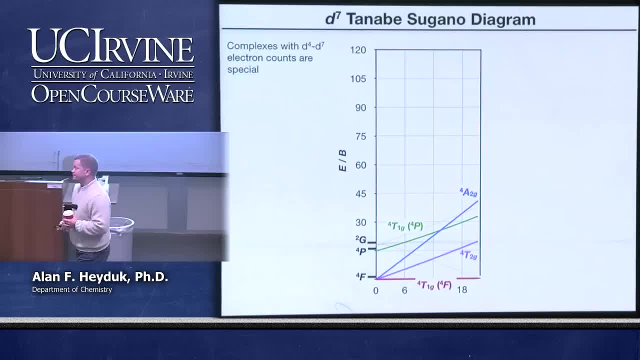 The Tanabe-Sugano diagram has to take that into consideration. And so if we consider D7, so if we have seven electrons, only five orbitals, we have two different cases. The first case is the high spin case. It's when you put all the electrons in so that you can. 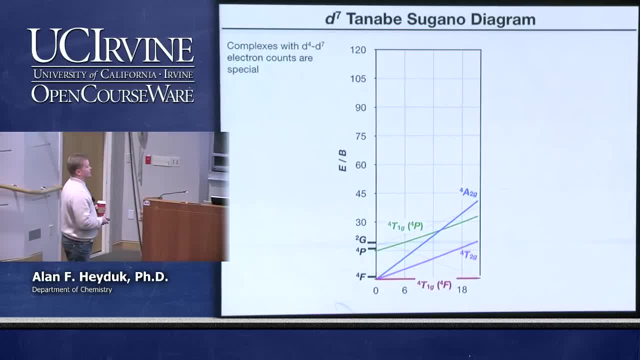 you can maximize the number of unpaired electrons. That happens when delta O is small relative to the electron pairing energy. It's going to happen right. so here's a Tanabe-Sugano diagram, or part of it, for the D7 ion. 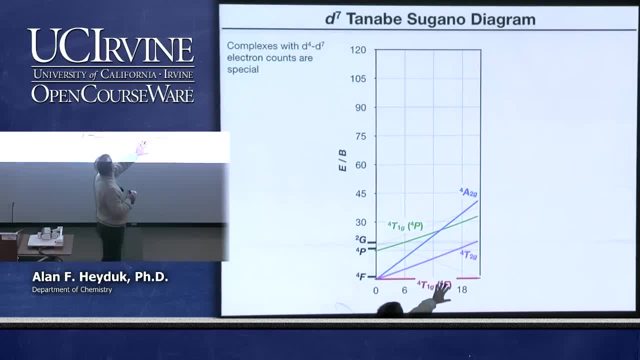 The X axis is delta O over B. Okay, So when delta O over B is a small ratio, yes, delta O of 5B or 10B or even 20B is considered a small ratio. you're in the high spin case. 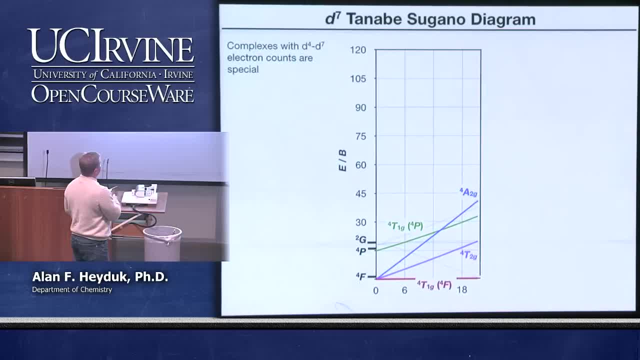 You have a ground state free ion term for D7 of quartet F. You have an excited state of quartet P. You'll notice, unlike the last time, I've included this doublet G free ion state. Right now it's kind of grayed out. 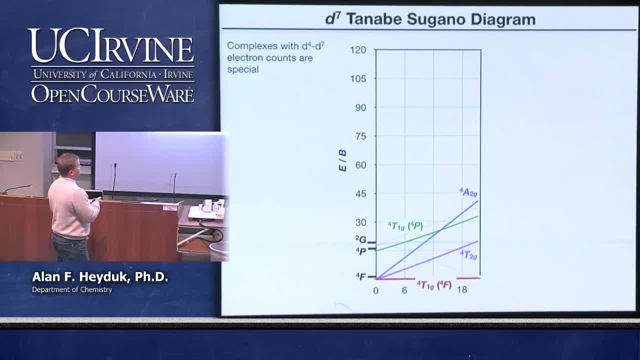 In the high spin case, the quartet F splits into and when we introduce octahedral symmetry, the quartet F splits into three different electronic states. The quartet P splits into three different electronic states. The quartet P becomes a quartet T1G. 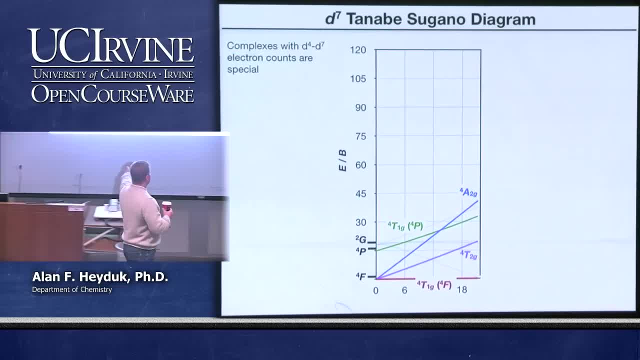 We go along This quartet. T1G is the ground state. What does it correspond to? Well, this is a D7 ion. Okay, We have five D orbitals. We're talking about the high spin case, So we put the first five electrons in all spin up. 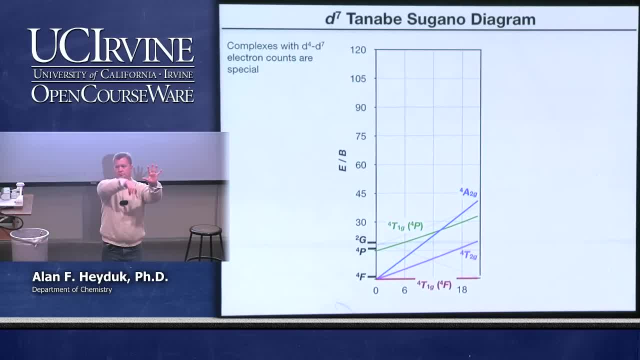 We have two electrons left over and they go spin down into the T2G orbital. So if you think about it, in some ways it looks similar to a D2 ion. We get the same three states here: T1G, a T2G and an A2G. 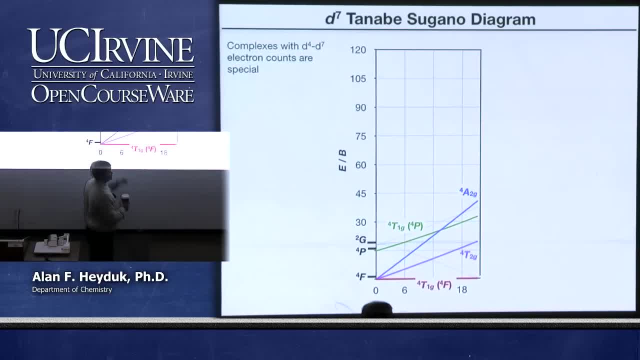 From an F state, the P state becomes a T1G. We're going along, We're increasing the strength of the ligand field, The states are splitting out in energy, just like we've seen before, until we get to this cliff. 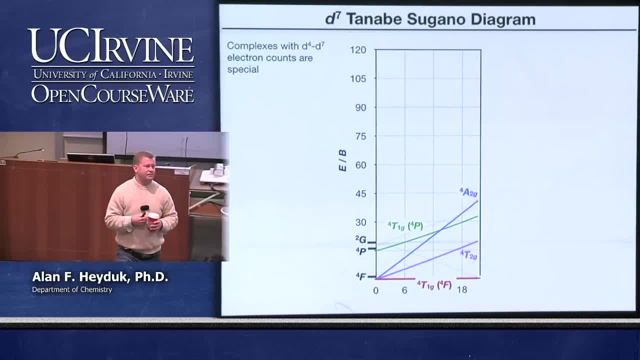 Now you could say, well, maybe D7 is just funny and delta O can never be bigger. Delta O over B can never be bigger than 18.. That's probably not the case, because if you have good eyes, you see that something else is happening. 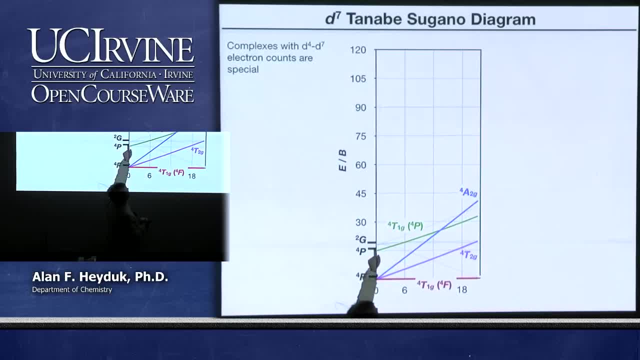 In this case I put the doublet G in here. It splits by the ligand field. but again, in a high spin complex we can't do a transition from a quartet ground state to a doublet excited state- Spin forbidden. 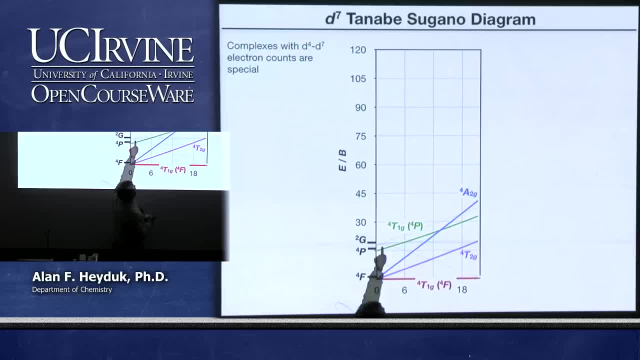 But nevertheless, as the octahedral ligand field increases, look, Here's the gray line. This is the lowest energy electronic state that comes out of that doublet G. It's coming down, it's coming down, it's coming down. 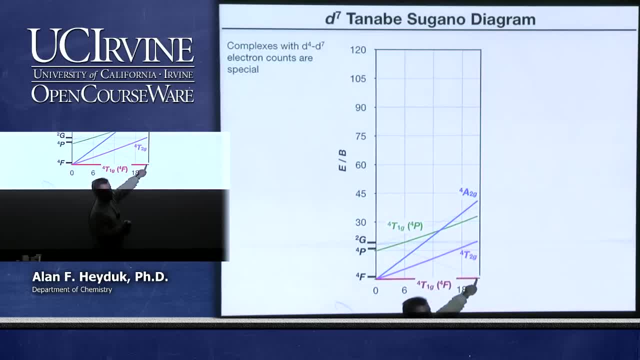 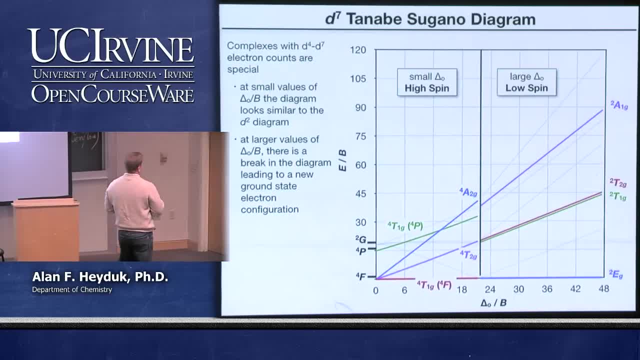 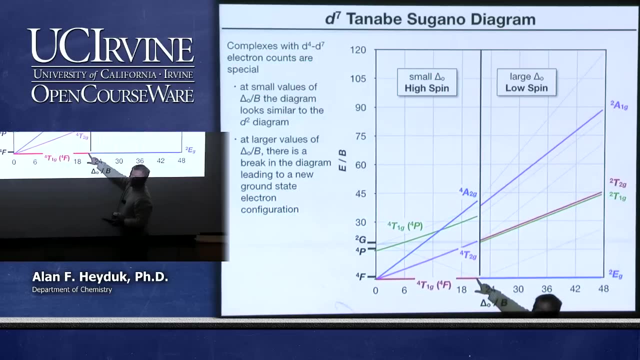 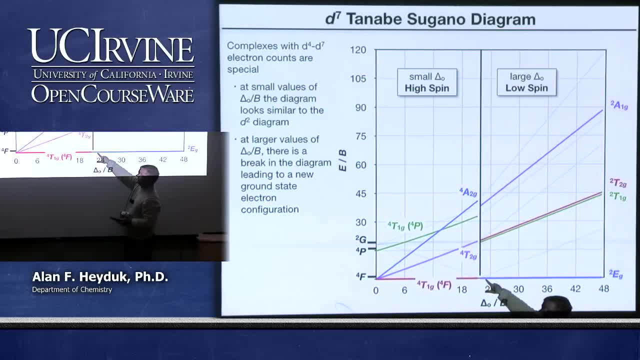 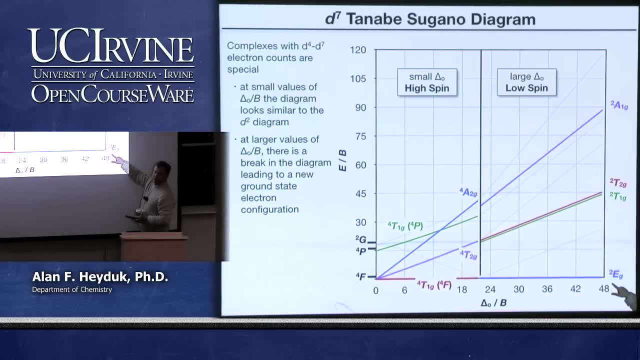 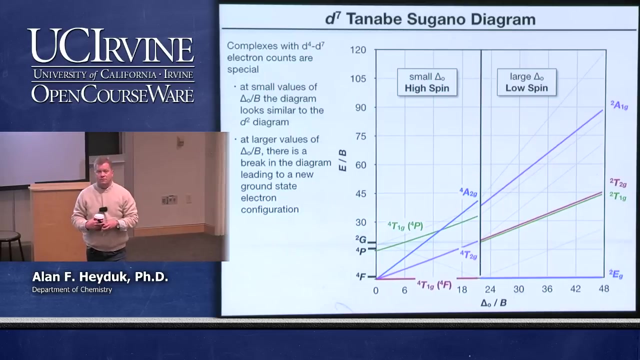 you transition from a high spin molecule to a low spin molecule And the state indicated by this blue line, a doublet EG, becomes the ground state. What does that doublet EG look like? Well, again we have seven electrons, five d orbitals. 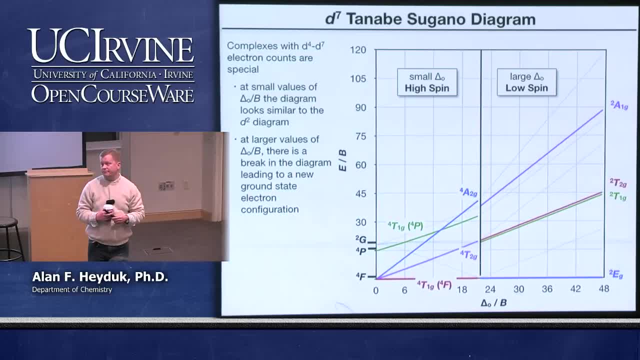 We put six electrons all paired up into T2G and we have one left over that goes up into the EG. That's the ground state electron confused with the ground state electron. So that's the configuration for a low spin D7 compound. 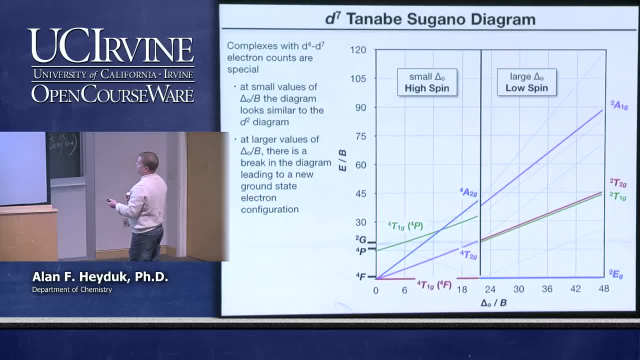 If the doublet EG is the ground state, we then have four excited states: a doublet T1G, a doublet T2G and a doublet A1G. that correspond to the excited states. Now, what happened? What happened to these quartet states? 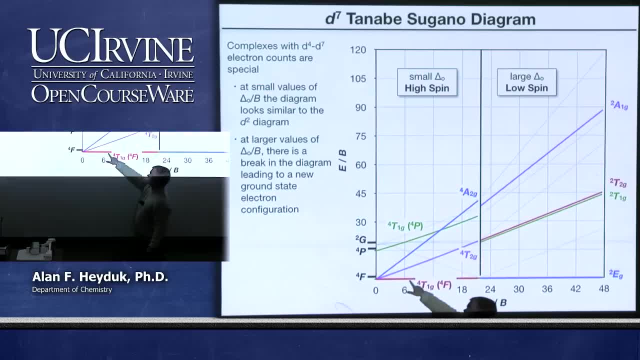 Well, we can see the red line was coming across, coming across as the ground state. We get to this crossing point and this red line starts going up in energy, because the energy of this state is now measured relative to this doublet EG ground state. 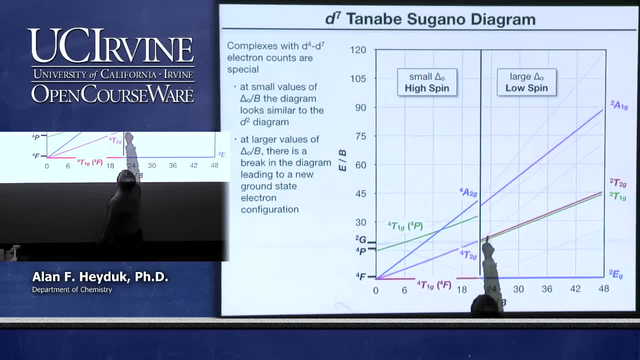 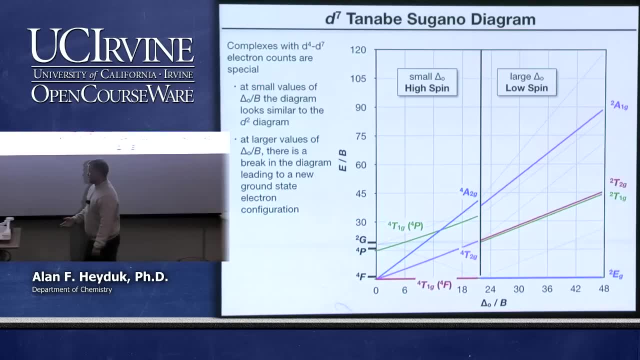 The purple quartet, T2G becomes that gray line that takes off in energy. You can correlate that, Correlate all of the quartet electronic states that are active in the high spin compound to states in the low spin compound which we can no longer see. 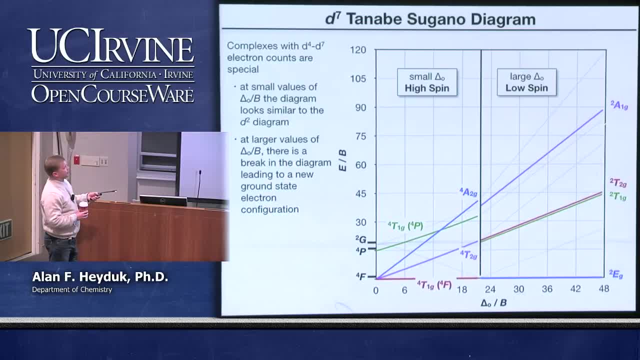 All of these electronic states, these doublet electronic states, come out of the doublet G free ion state. All right, So we're going to go ahead and do a little bit more of this. So we're going to go ahead and do a little bit more of this. 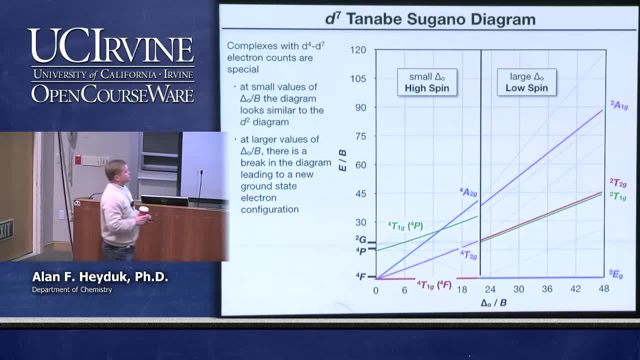 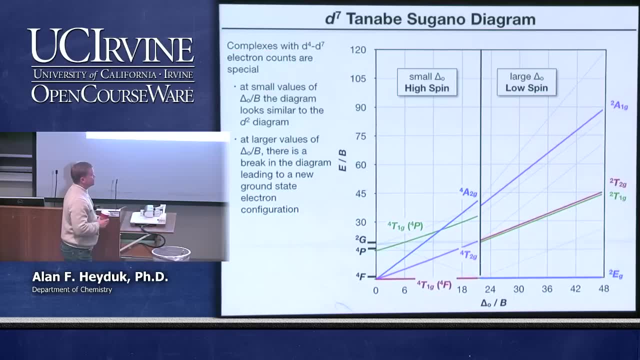 So we're going to go ahead and do a little bit more of this. The position of this break is consistent for any D7 ion. Okay, It's going to occur. it's right around 21 or 20 delta O over B, But of course, the magnitude of delta O 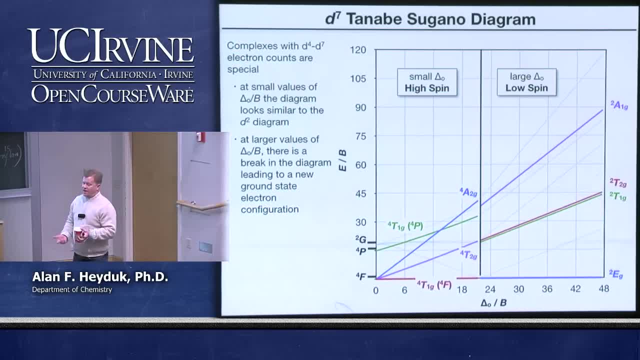 and the magnitude of B are going to change depending on the metal ion, the ligands, so on and so forth. Yeah, Good question, Right? So on the left-hand side of the diagram it looks like a situation where we should have one. 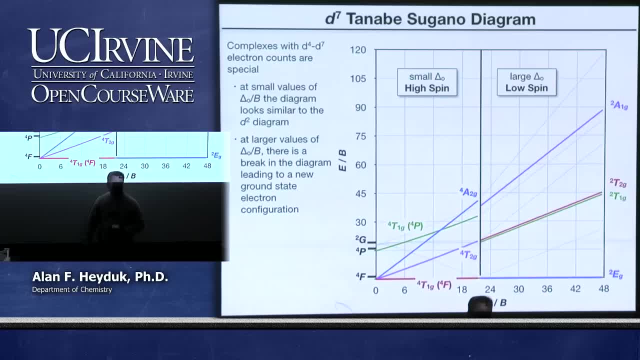 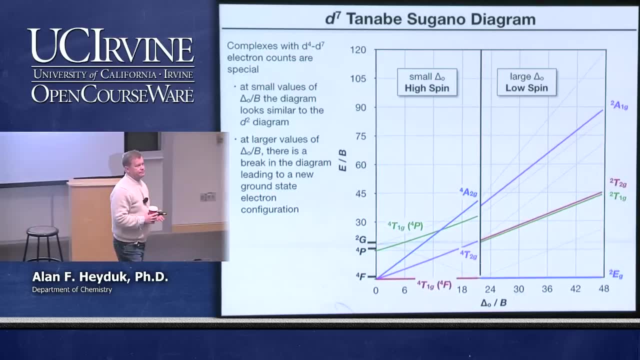 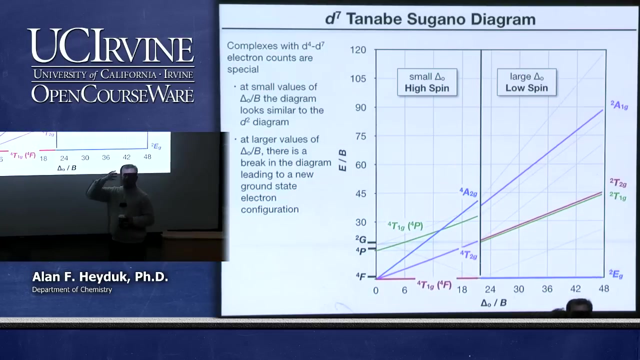 two, three transitions, And that's what you nominally will see for a high-spin, D7 ion On the right-hand side. for the low spin, we clearly have three excited states And so technically- yes, you're correct, There should be three transitions. 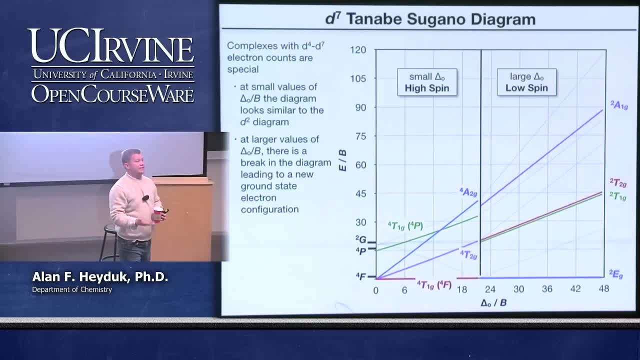 in the visible region that we can ascribe to D to D transitions, to these three different excited states. Now, that's technically In the real world. we have certain issues with doing experiments, one of which is resolution, Right Resolution. how close can two things be? 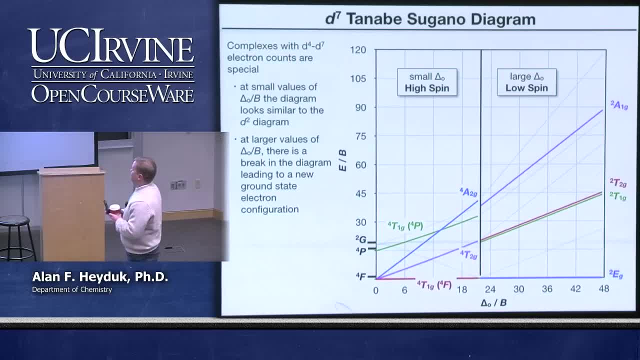 where you can still separate them, And what we observe is that the transition from the ground state to the doublet T1G and the ground state to the doublet T2G. we can't resolve those, So they because they appear so close in energy. 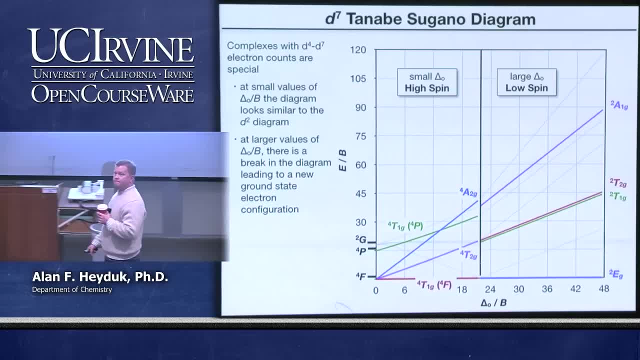 that we just can't see the difference. Yeah, So then you can tell if it's high spin or low spin based on the absorption spectrum, That's. that's yep in, with the caveat right, because you could go through back to this side and say: 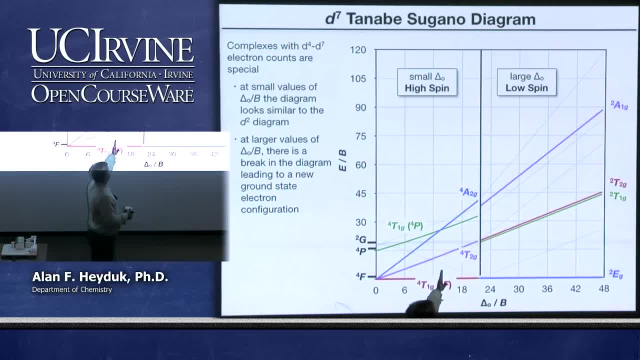 well, what happens if my delta O over B value is right here at about 14?? And we end up with the same problem. It's a resolution We can't right because these two are crossing right here. we're not going to be. 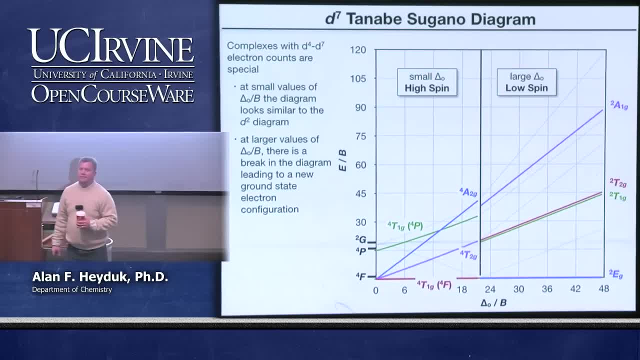 we're going to see two absorptions rather than three, And so, but yes, that the whole point of this is that the electronic absorption spectrum can tell you exactly whether it's a high spin or a low spin compound, assuming that you know, you have a little bit of luck and you know how. 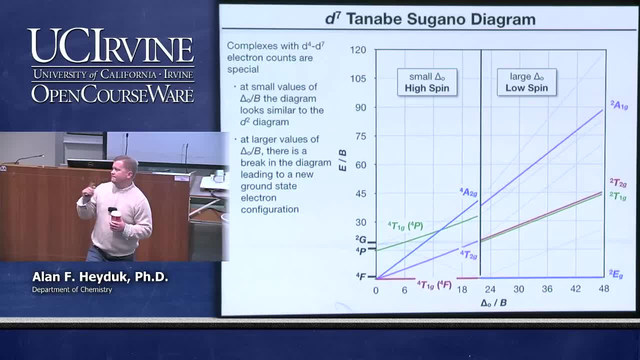 to analyze that, Right. So that's the problem. Yeah, Wouldn't it be better to look at the wavelength of where it absorbs, Because the ones that are lower in energy are going to have a larger wavelength. The ones that are lower in energy are going to have? 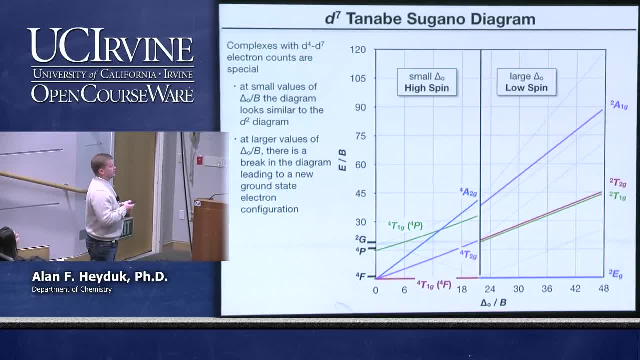 Because that's going to have a lower energy transition, so it should be higher wavelength. Yes, So in general, that's true, You're going to have higher energy absorptions- D to D absorptions for low spin compounds- than you do. 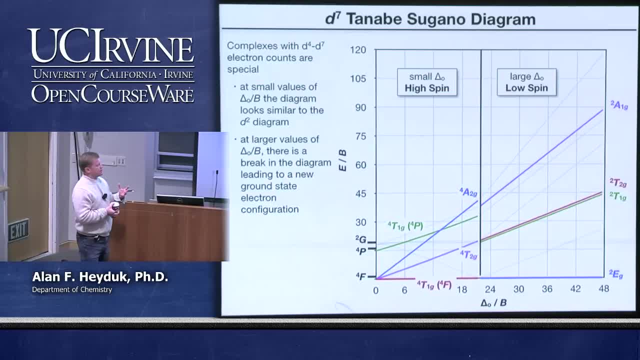 for high spin compounds, Though remember, on this diagram what we're looking at is delta O over B, And so if B is larger, that can force the ratio smaller. Right It's. the important thing for high spin versus low spin is the magnitude of delta O relative. 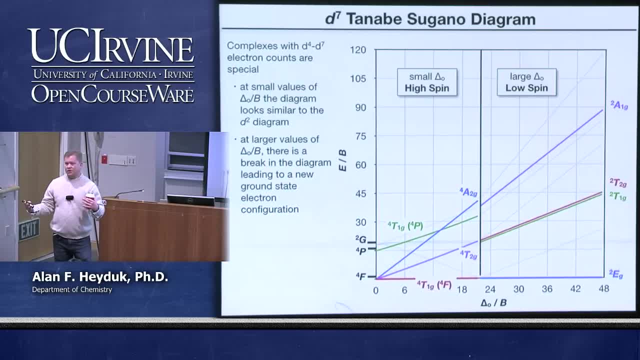 to the magnitude of the electron-electron repulsion. So in a small ion the electron-electron repulsion can be higher, And so that can muddle things. The other problem of course that you run into and again 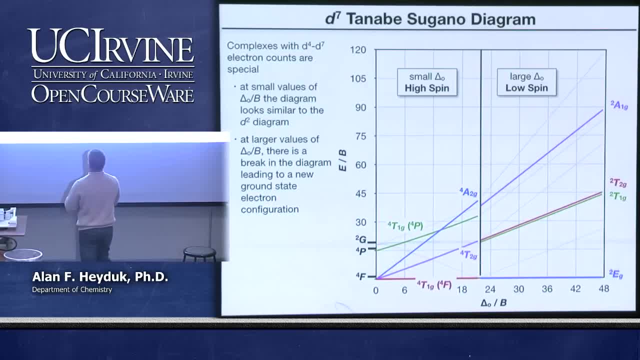 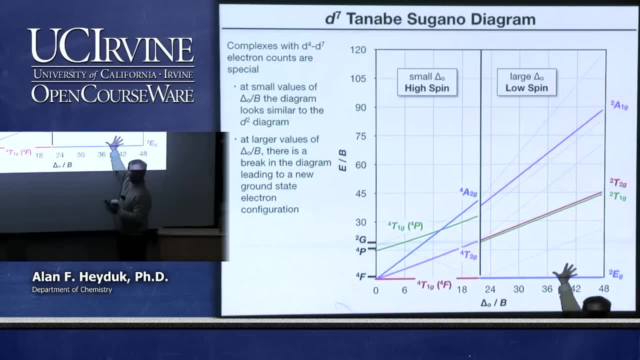 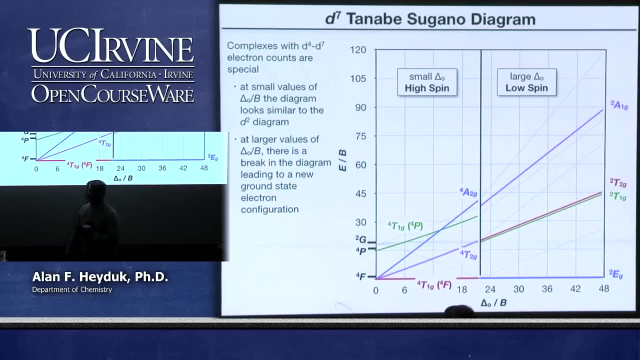 this is everything in science seems to be this way. There aren't a whole lot of complexes that lie over here, And there aren't a whole lot of complexes that lie over here. However, there's a ton that lie right around here. Okay, Where you're playing on either side of the line. 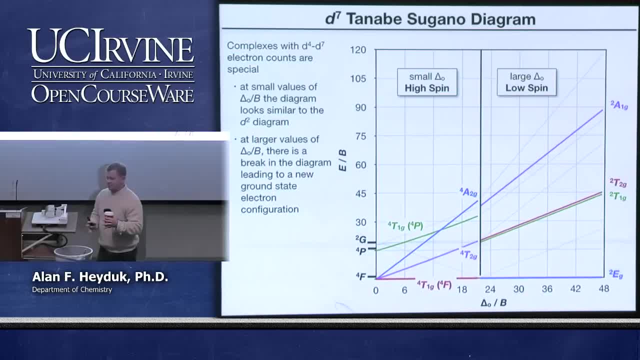 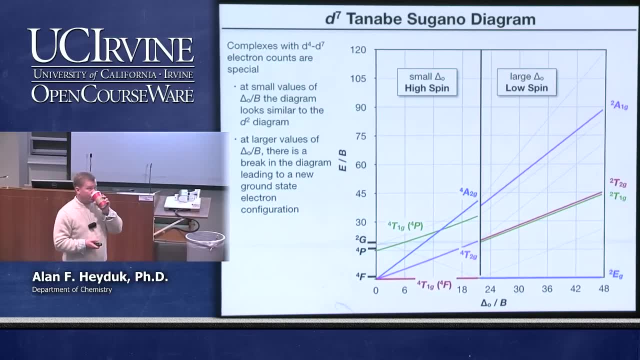 and it becomes difficult to know exactly. Okay, So that's the problem. Yeah, So that's the problem. So that's the problem Exactly. the magnitudes end up looking very similar. Any other questions? So if you look in the back of your textbook, 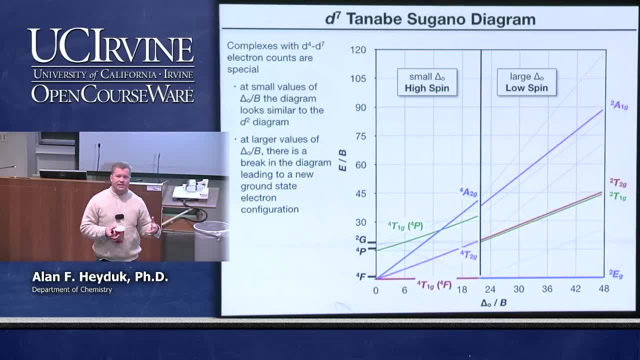 the Tanabe-Sugano diagrams for octahedral complexes in every possible electron configuration are known. Okay, There's also a relationship where the D2 looks just like the D8, the D3 looks similar, looks similar to the D7, except for the whole high-spin. 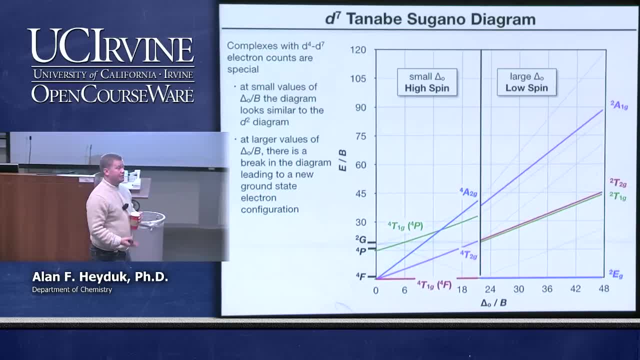 low-spin thing A given Tanabe-Sugano diagram is. really it's very sensitive to the geometry. Okay, So the ones that you have in your textbook are all for octahedral complexes. If you read the chapter in your textbook, 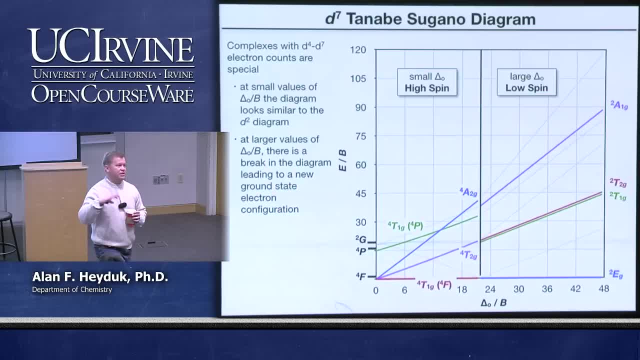 which you should be doing. it'll tell you there's a relationship between an octahedral- Tanabe-Sugano diagram- and a tetrahedral. they're kind of inverted from one another. You should be able to convince yourself that that should be true, because the MO diagram looks. 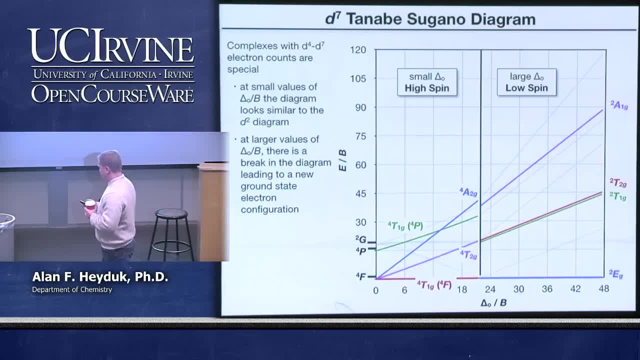 like of a tetrahedron, looks like it's inverted from an octahedron, But certainly if you go to a different geometry then the way these electronic states split from the free ion changes and it becomes a more complicated problem. 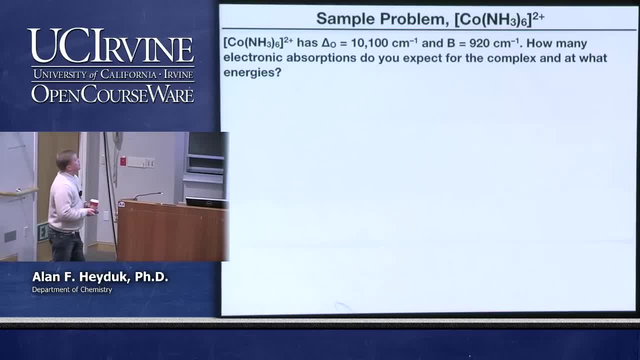 Okay, The promised sample problem, Hexamine cobalt dicat ion, has a delta O value of 10,000 wave numbers and a B value of 920 wave numbers. How many transitions and at what energy do you expect to observe them? 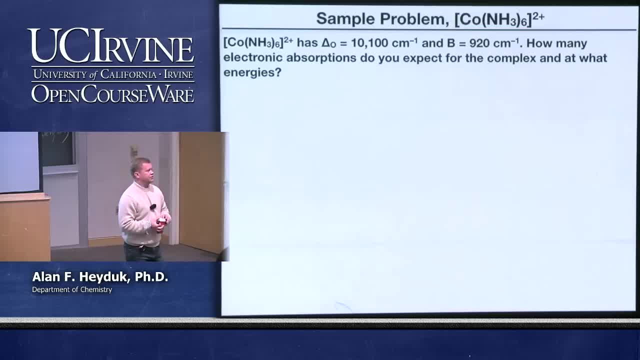 Okay. So again, this is kind of a backwards way to do the sample problem, because if you were to actually go into the lab and make a measurement, you would measure the transition And you would want to calculate delta O and calculate B. 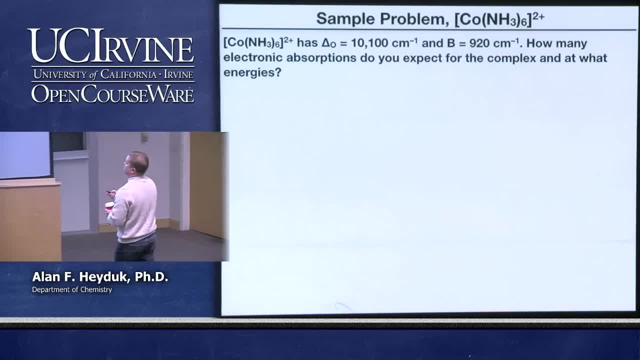 But for the first pass we'll go through it in this backwards way where we're giving you the delta, O and the B value. It's a good problem because it means we have to figure out the oxidation state for our cobalt. 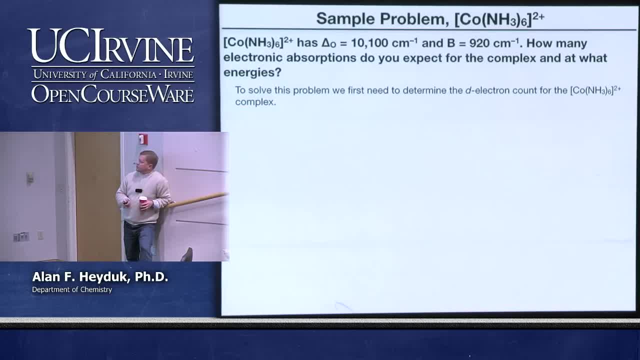 and how many D electrons it has. So this is a good freshman chemistry problem. We know that we have six ammonia ligands on the cobalt. they're all neutral Lewis bases, So we can basically just remove those and say that we have cobalt with a plus two charge. 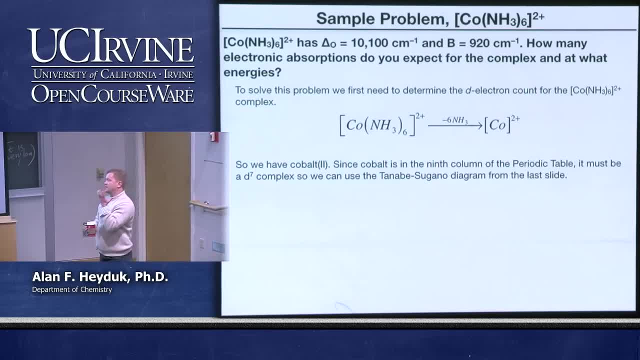 We know that cobalt is in well, the ninth row of the periodic table, seventh row or seventh column of the transition metal series, so it must be a D7 complex. Once we have the electron count, we need to calculate delta O. 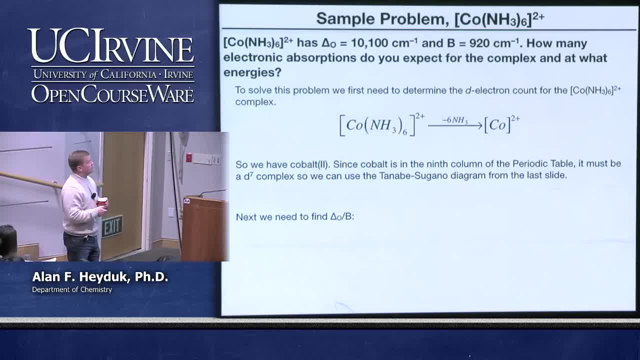 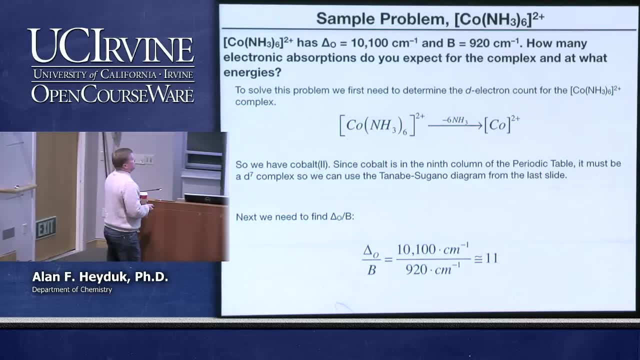 over B. Conveniently it's D7, since we just got done looking at the D7 Tanabe-Sugano diagram. So simple math: 10,000 wave numbers divided by 920 wave numbers gives us a ratio of delta O over B. 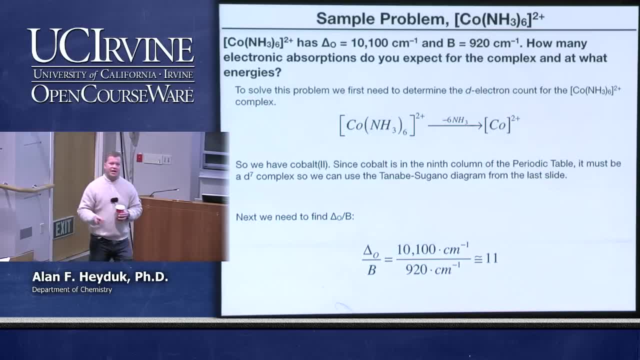 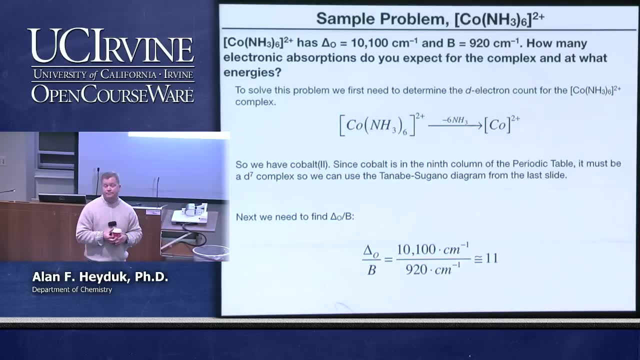 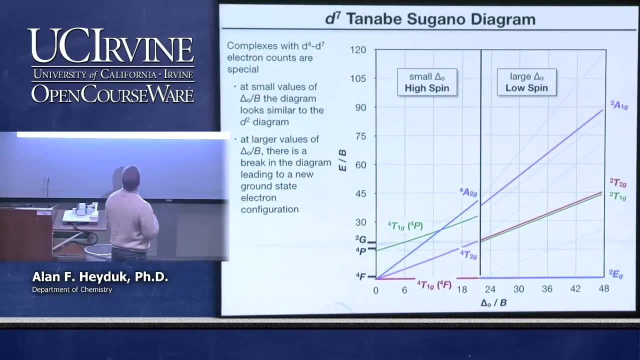 of about 11.. So, since we just finished looking at the D7 Tanabe-Sugano diagram, we remember that that pretty much puts us in the high spin configuration. Well, what happened there? Okay, so here's our Tanabe-Sugano diagram. 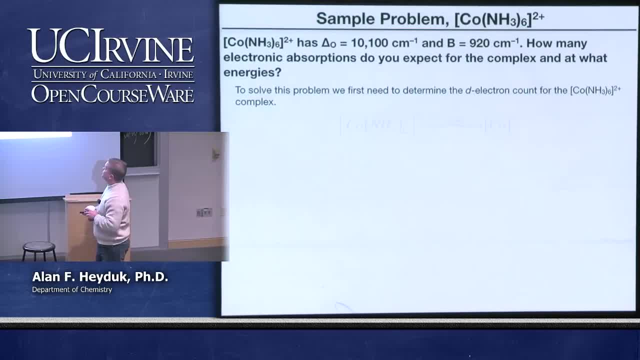 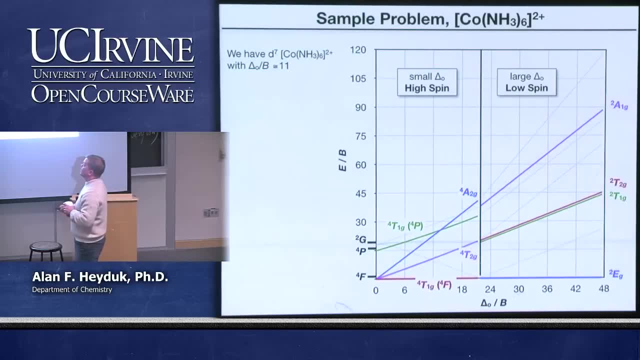 What the heck? Oh, It would help if I hit the forward button instead of the backward button. That's the problem. Okay, Looks the same. Okay, So we have a D7 ion with delta O over B is equal to 11.. 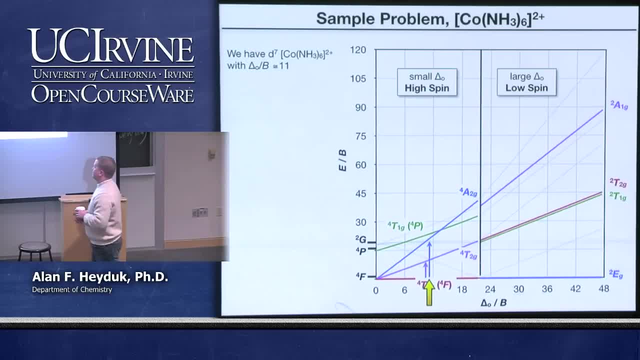 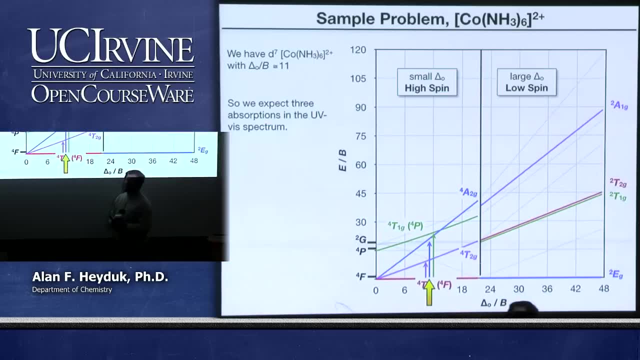 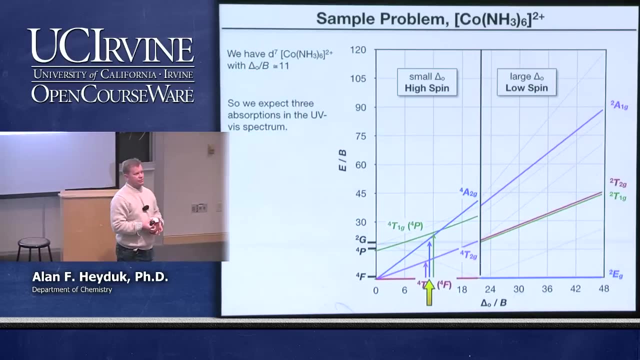 We come to our Tanabe-Sugano diagram and we say that delta O over B of 11 is about right here, And so we can expect to see three transitions, assuming that we have a spectrometer that has suitable resolution to differentiate between the blue and the green arrows. 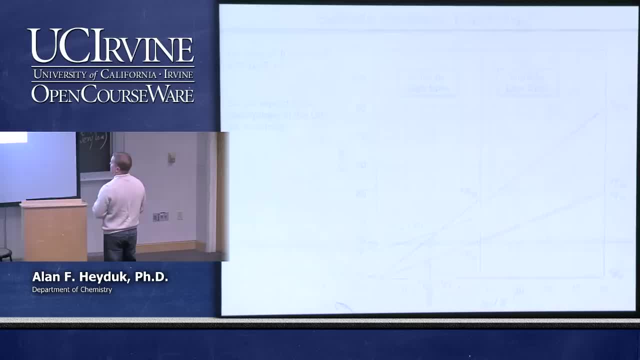 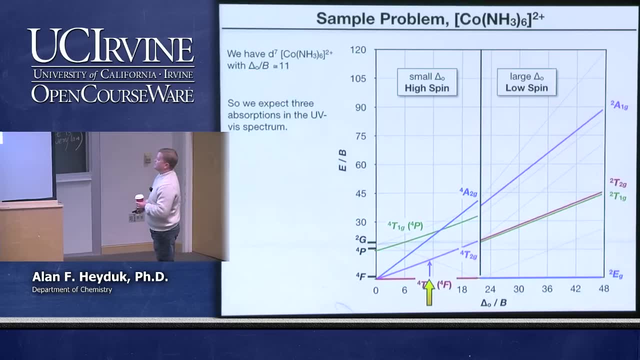 shown on this slide. The first transition is from the quartet T1G to the quartet T2G. We can come horizontally across and read off, And if we look at the diagram we can see that E1 over B is going. 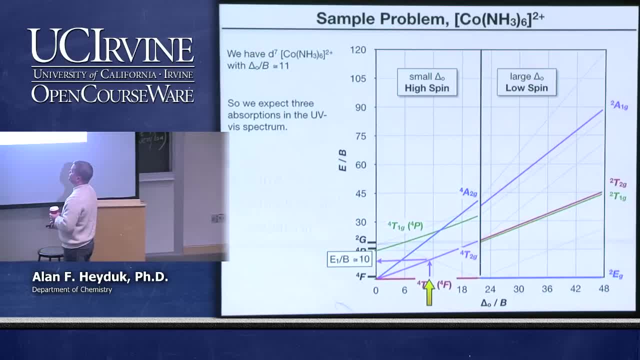 to be approximately equal to 10.. From the problem we know the value of B. it's 920 wave numbers. So 10 times 920 wave numbers tells you that the lowest energy transition should appear at about 9,200 wave numbers. 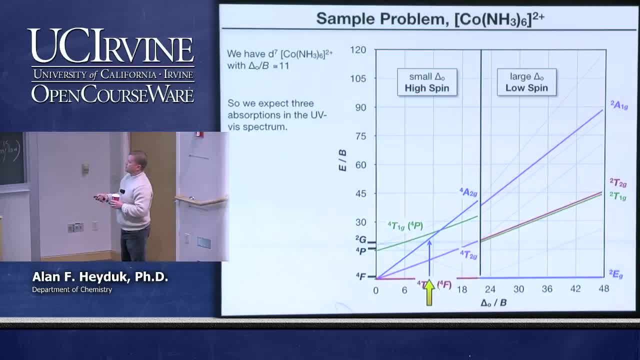 The second transition is going to be from the quartet T1G, in this case, to the quartet T2G or, sorry, quartet A2G. So that's kind of interesting, because it's telling you that the electron configuration where we move two electrons is: 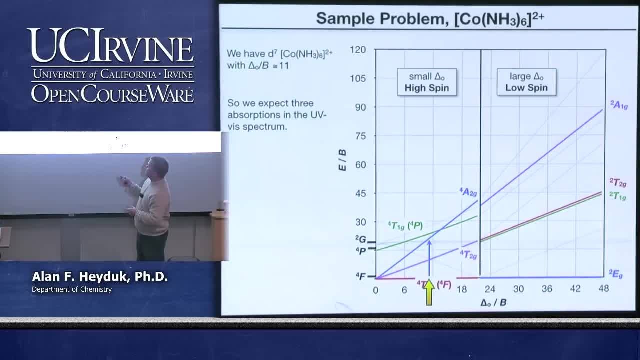 lower in energy than this quartet. T1G. Right, Because this gap here is effectively 2 delta O. But again we come across to the Y axis. In this case E2 over B is 18.. Eighteen times 920, wave numbers tells you. 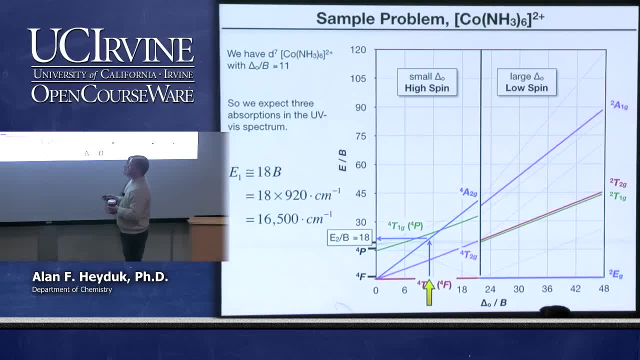 that this transition will be observed at about 16,500 wave numbers. We calculate the energy of the third transition in the same way. That should be at E2,, by the way, E2 is equal to 18B. The third transition is to that, to the state indicated. 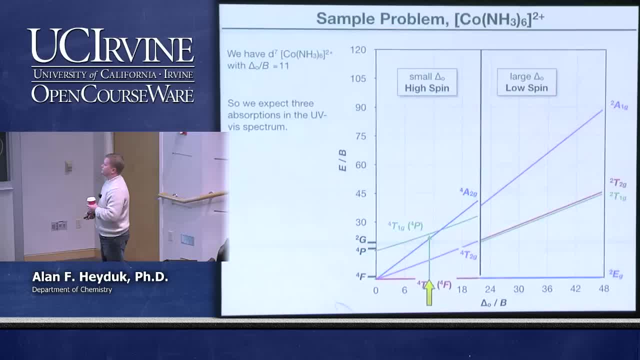 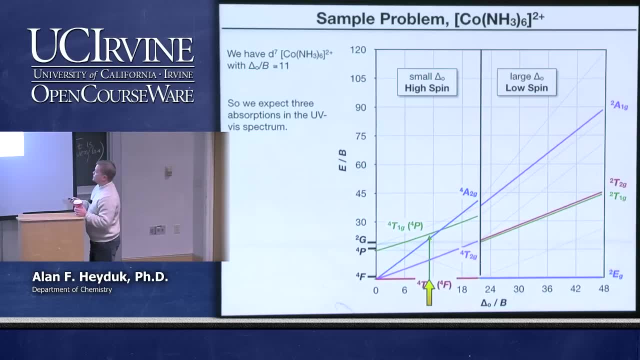 by the green line, the quartet T1G. Again, this is probably- it's probably going to be hard to resolve this problem Right. This transition is separate from the one to the blue quartet A2G state, But we can calculate it, of course. 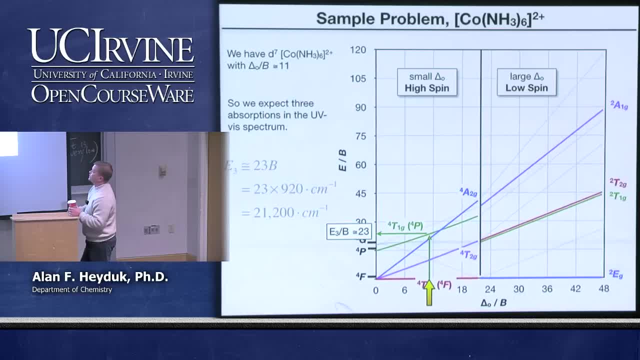 In this case, E3 over B is about 23. And we calculate that that's that the energy of the third transition should be at about 21,000 wave numbers, That's probably about 480 nanometers. Okay, So we've seen now how to go. 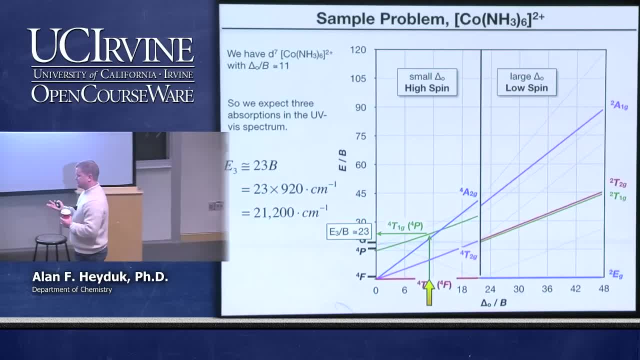 through and calculate. we would calculate the presence of three transitions based on the state diagram or the Tanabe-Sugano diagram, And we can estimate the energy at which they come through. If you take this and divide by 2, you should get about delta O. 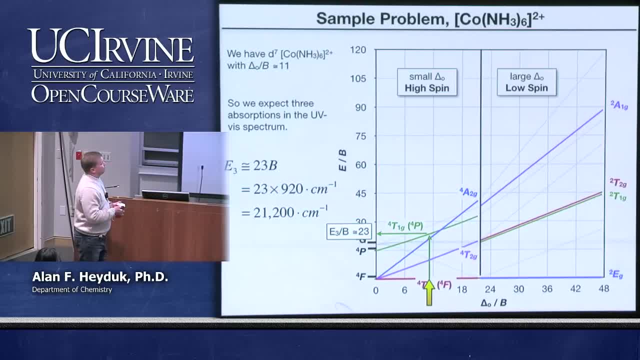 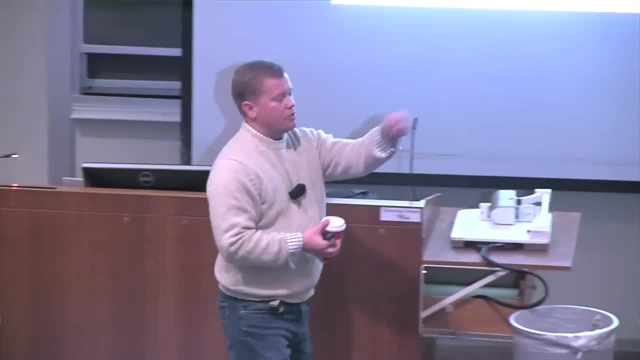 Actually sorry. the previous one should be about delta O, And so you can correlate those to the to the appropriate electronic states. We will stop here. cover Jahn-Teller distortions on Friday, along with electron counting. Have a great day.